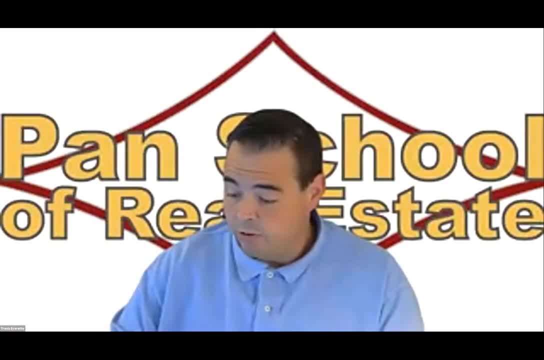 Law. So the natural sort of follow up to landlord tenant law is property management, And that's what we're going to cover right now. And this is this is one of the shorter chapters, and I told you in the second half of the class There were quite a few chapters that are really, you know, a lot shorter, And this is one of those and we'll get you'll, you'll see quite a few of those. This is one of those shorter chapters. 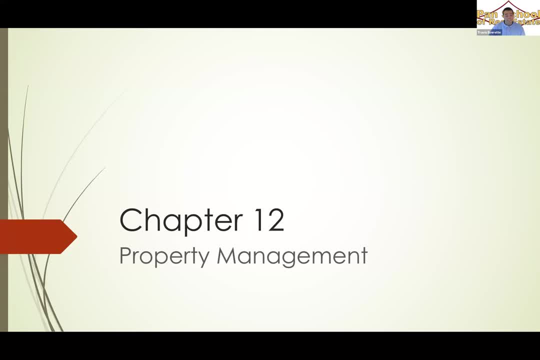 Then chapter 16 is super short: basic residential construction. chapter 18, which is taxation, is short. The environmental chapter is super short. So there you know, there are quite a few chapters left to cover, but you'll be shocked at how quickly we'll click off several of them. 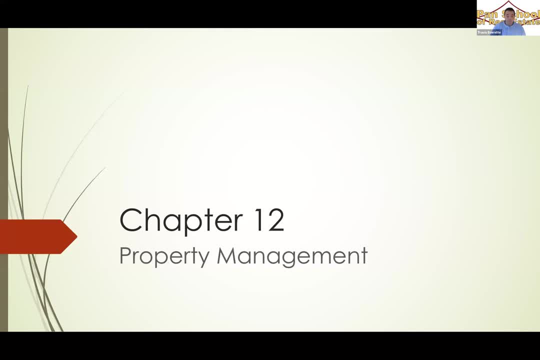 There are some heavy duty chapters left. So for next week you really need to spend some time getting ready for the finance chapters and valuation. But You get down to the point where you don't have a lot of heavy information left, So that's a good thing. right here, Almost you know your brain is almost full right, are y'all like? full up at the top? You got a little bit more. We have to cram in there. 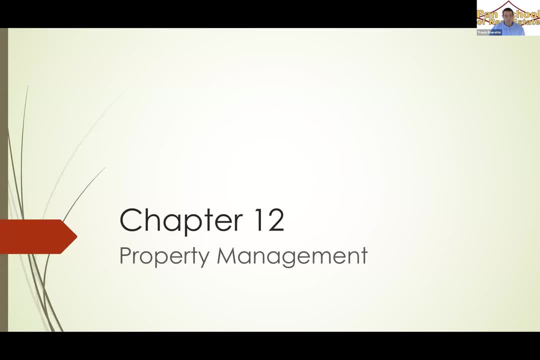 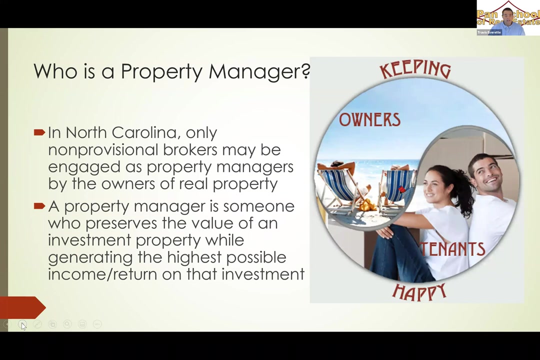 So property management is the brokerage service that we render to landlords. when we represent sellers, We call that listing. When we represent buyers, we call that buyer agency, and we represent landlords, we call it property management. And property management is a little bit different than the other types of agency that we talk about, because property managers have more authority. 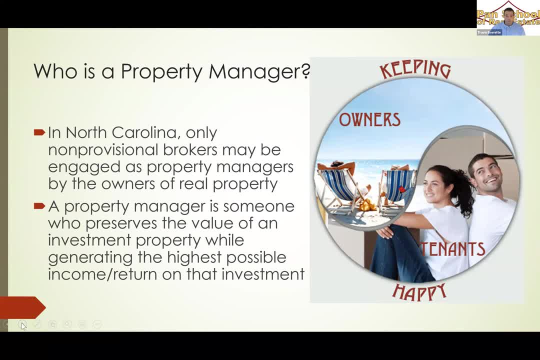 To make decisions than we do as agents when we're working for buyers or for sellers. property managers are expected to manage to actually make the decisions about a number of things. One thing to know specifically about North Carolina: look at this part of this statement here. It says: 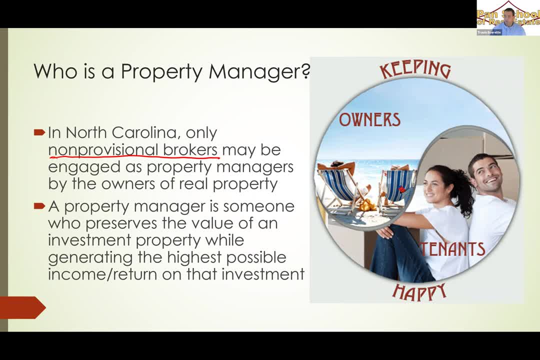 only non-provisional brokers can be engaged as property managers. Now that does not mean a provisional broker can't help with property management. They can. They can work on property management accounts, but they cannot be the property manager. And the reason: a provisional? 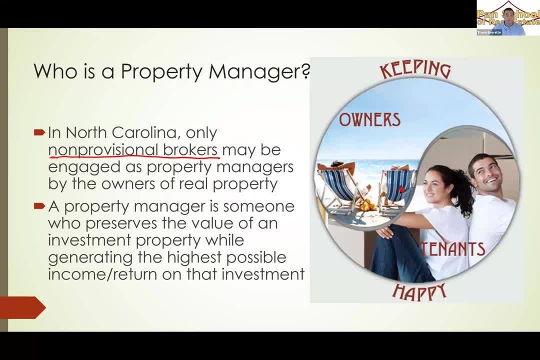 broker can't be the property manager is because of that decision-making. Property managers are expected to make the decisions on how much to charge for rent, what tenants to accept, whether or not to evict a tenant, what maintenance to do on the property. All of those are decisions. 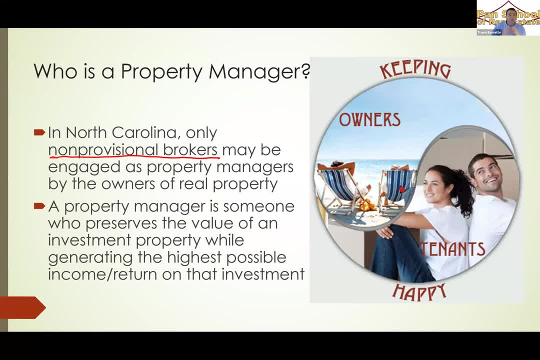 that sometimes lay with the property manager. We don't want to give that much decision-making money to the property manager. We don't want to give that much decision-making money to the authority, to a provisional broker. So what we say is that if you're going to serve as the property, 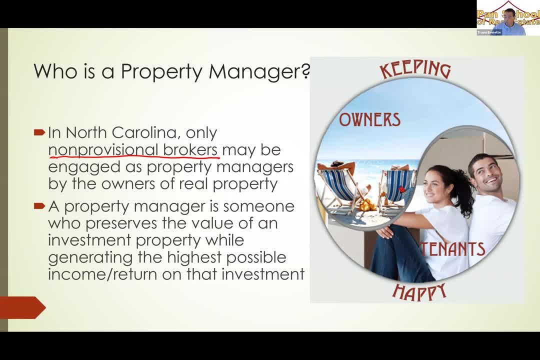 manager, the primary property manager for a property. you need to be non-provisional. The purpose of a property manager- if you're asked on a test- is to maintain the value of the property while generating the highest possible income or return for the property's owner. 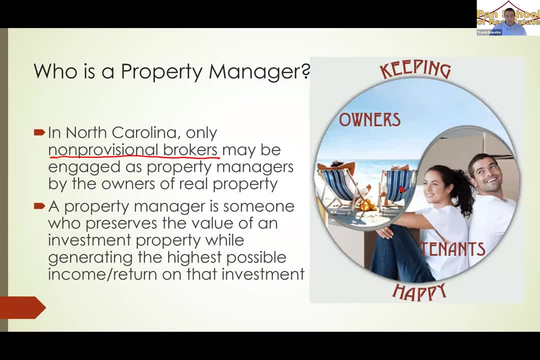 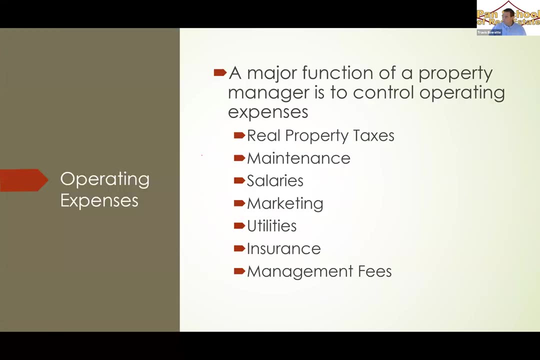 Basically, you become like the property owner: You're looking out for the best interest of the property, What is in the best interest of the property both right now and long term. And that's where the maintenance part comes in, That long-term sort of looking after the. 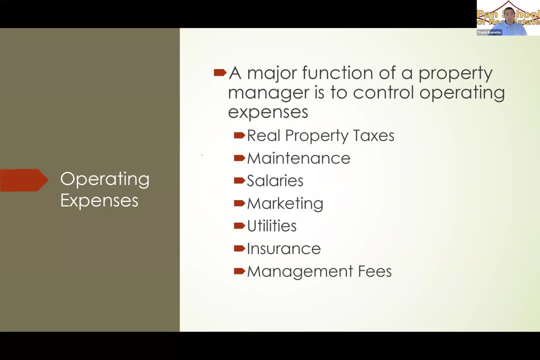 property. One of the terminologies that you're going to have to familiarize yourself with for the property management section is: what is an operating expense? Operating expense is when you're trying to make money off of something boxed in, Like if you're a landlord. 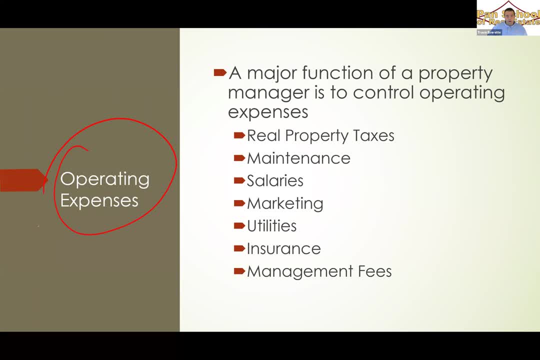 expenses are basically everything that a property manager would spend money on. You name it. If the property manager is spending money on it, it's an operating expense. The property taxes like the real property taxes every year. if you're managing property, that's an operating expense. 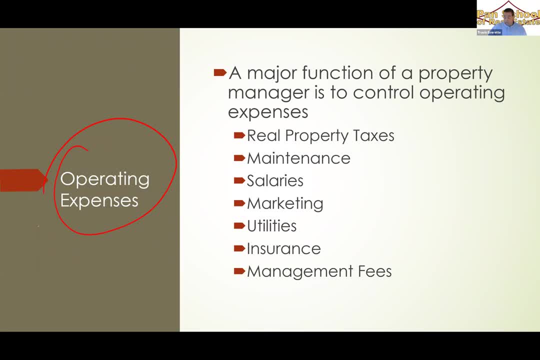 The maintenance that you do on the property, that's an operating expense. Any salaries that you pay If you pay a property, if you pay yourself a property management fee, that's an operating expense. Utilities insurance on the property- all of that falls in this one big bucket. 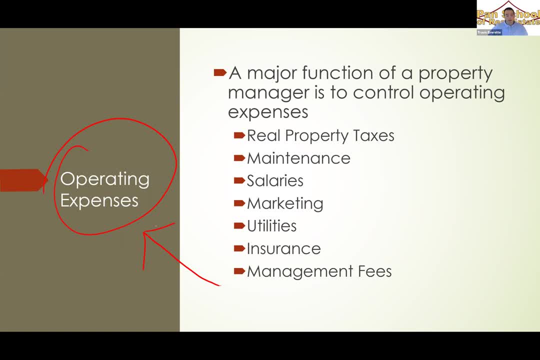 of operating expenses. But I'm going to point out one thing that's not on this list and we'll write it here in a different color. One thing that is not on this list: mortgage payments. Could these properties that we're managing for these owners? 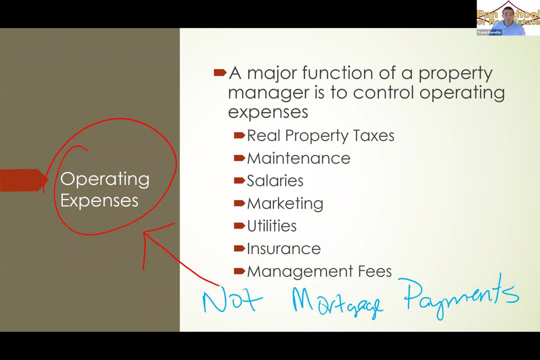 have debt. In other words, could they have a mortgage on them? Yes, Absolutely. Very commonly they do. This is the one check that a property manager would write that's not going to be considered an operating expense. You need to know that for the test. So not mortgage payments. 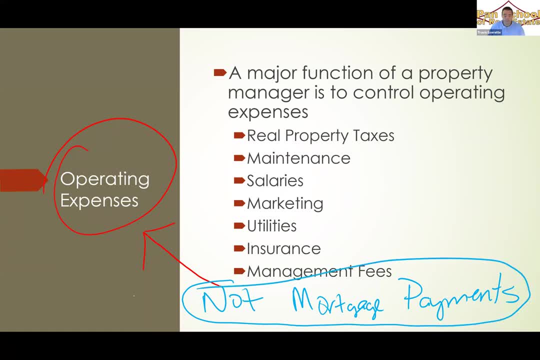 Everything, Everything else that a property manager spends running that property except- and another word for mortgage payments is called debt service, Debt service. You are servicing that debt That's not going to be considered an operating expense. I have a question. 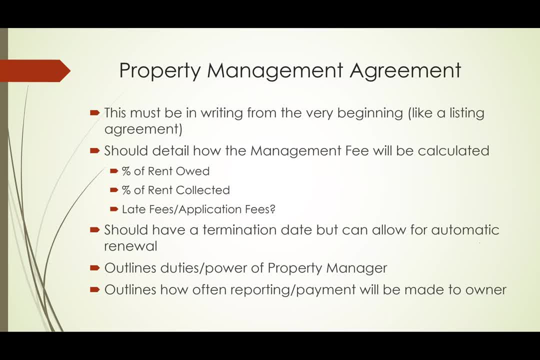 Okay, go ahead, Justine, Because I'm in property management and it's kind of on the first slide that you did about the non-provisional, because I've seen some companies that require you to have your real estate license, but I've also seen some that they 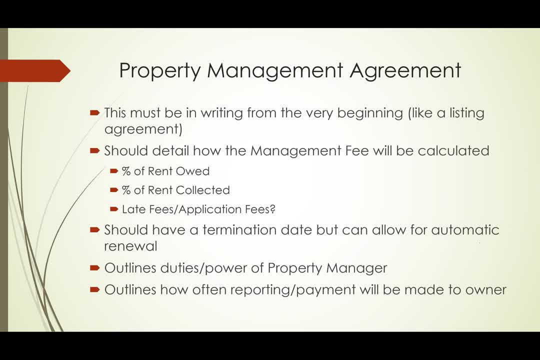 don't want you to have it. Is it based off of where the property management company itself is out of or where the property is at? It's where the property is located. but remember also there's no requirement that a property manager be licensed at all if they are salaried. Remember. 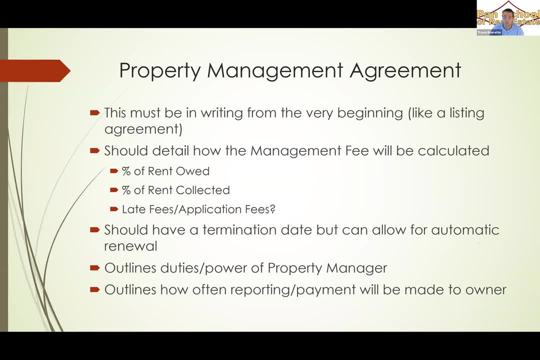 one of the exemptions to the licensure rule is the salaried employee of the owner of the property. So a lot of property managers are not actually licensed at all And they have trust accounts even if they're not licensed. Yes, you do not have to be licensed to have a trust account. Anybody can open a trust. A trust account is just a checking account. 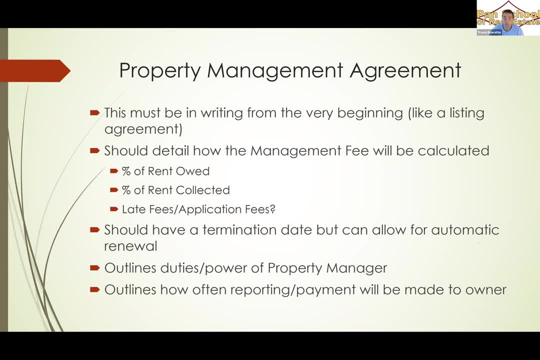 That's all it is. It's just a checking account, Okay, Where you keep other people's money- Yeah, separate from your own money, and you just label it as trust account to clearly tell everybody: this is not my money. did that help answer your question, justine? um, it does a little bit i. i've only seen. 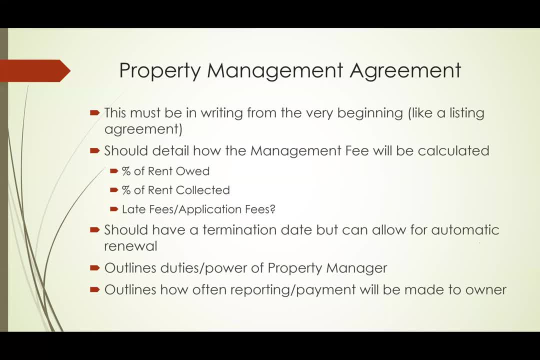 like one company. it was a company that i had interviewed for um at the beginning of the year and they required all of their employees to have their real estate license. so that's why i was like, and that's just an interior, yeah, that's just an internal decision based that they decided that. 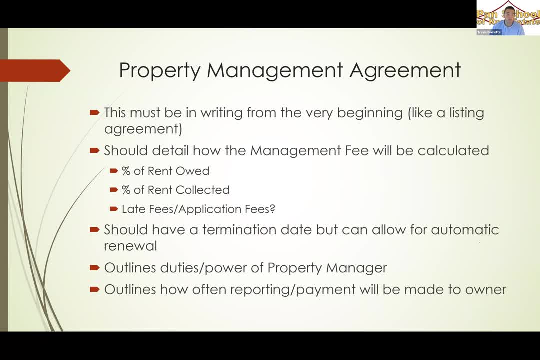 they could have gone the other route. if their employees, if their w-2 salaried employees, they could have hired unlicensed people. but that's their choice. they don't have to be licensed. okay, i got you good, but some choose to have. if i was hiring property managers, i'd want to hire. 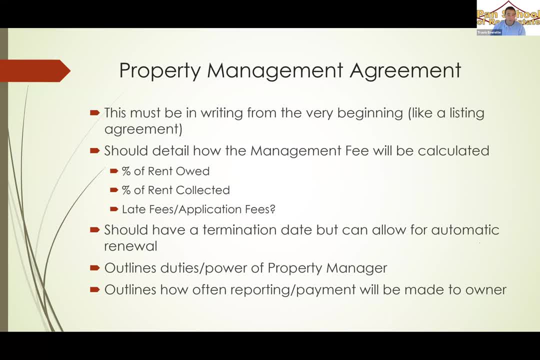 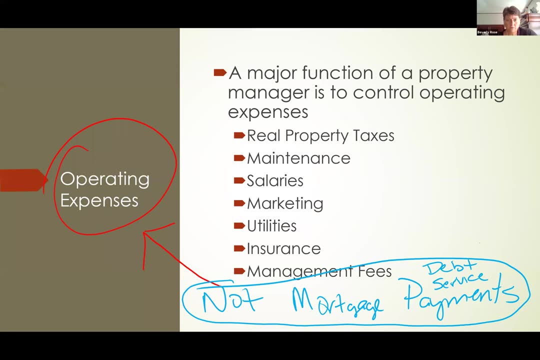 lots because i'd be less concerned they would make mistakes, i'd be more comfortable, they knew what they were doing. so you, Travis, can you back that one slide for just a second? sure, that way that's all right. okay, thank you, yep, yep. so basically, on that slide, everything that a property manager would spend money on. 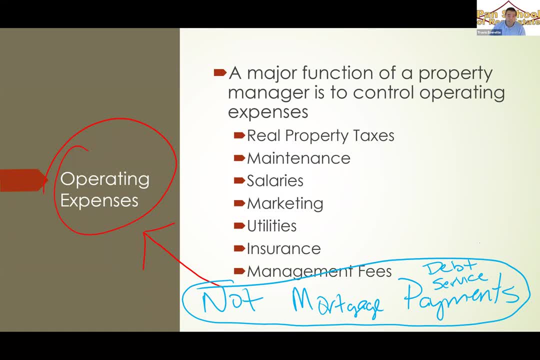 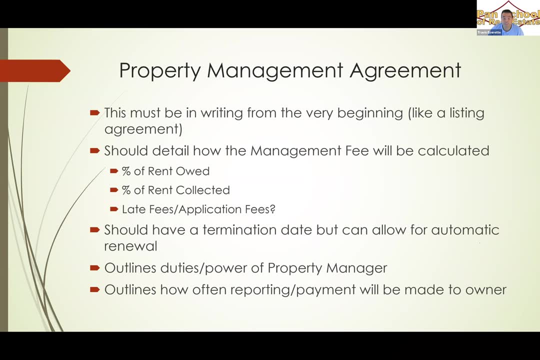 is an operating expense, except any debt service or mortgage payments. okay, now, as far as the agreement, remember, we always need an agency agreement. we can't get paid unless we have what kind of an agreement with our client? a written agency agreement, a written agency agreement. we need a listing agreement if we're 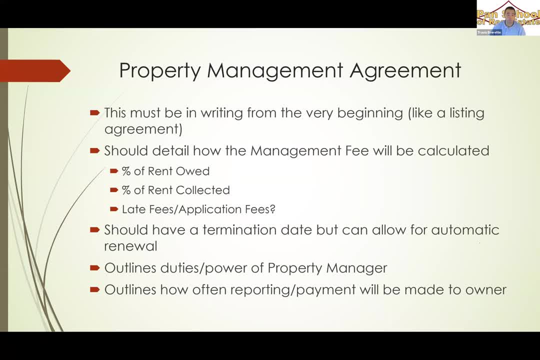 going to represent the seller and get paid, we need a buyer agency agreement if we're going to represent the buyer and get paid. if we're going to um represent a landlord and get paid, we need a property management agreement. it's got to be in writing, otherwise we don't have any entitlement to. 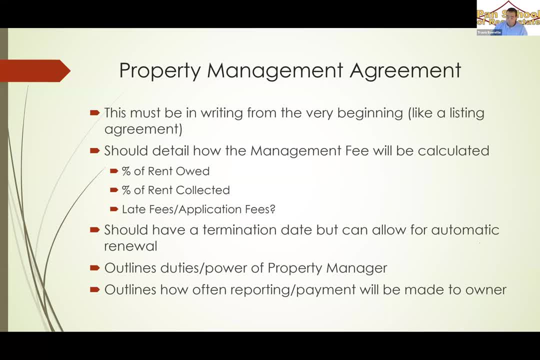 compensation. um. one of the things that's most important in the management agreement is um how much power the property manager has. in other words, can the property manager decide on maintenance, or do they have to go to the landlord every time? that that should be in the property management agreement can. 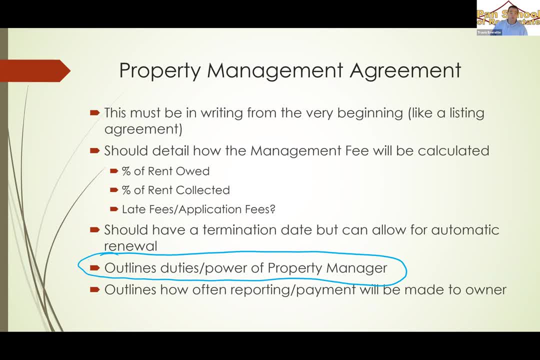 the property manager decide to evict a tenant, or do they have to go back to the landlord every time? that should be in property management agreement. the other thing that's important to put into the property management agreement is: how are we we going to calculate our fee? How are we going to calculate the amount of money that we owe, And so? 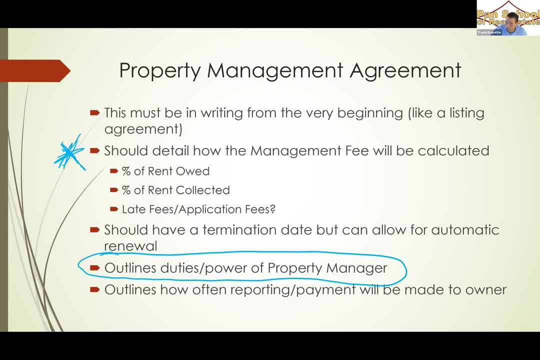 how should the fee be collected or calculated? The most common method is a percentage-based method, sort of like the sales commission. but the percent of rent collected is the most common percent of rent collected. Why do you think percent of rent owed is not as much is not as. 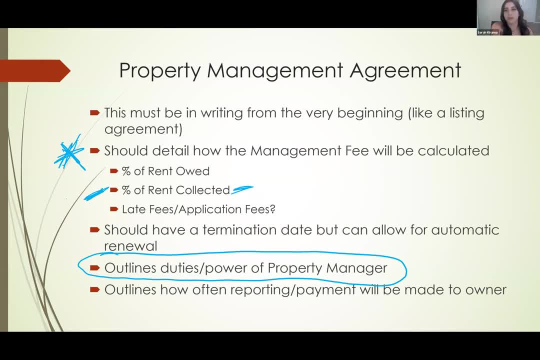 common as percent of rent collected. Not everybody pays their rent, Not everybody pays their rent and the property owner doesn't want to pay us for rent. but we did not. That was not paid. We did not get paid Exactly. Okay, The other thing that the property management agreement should make a point of: 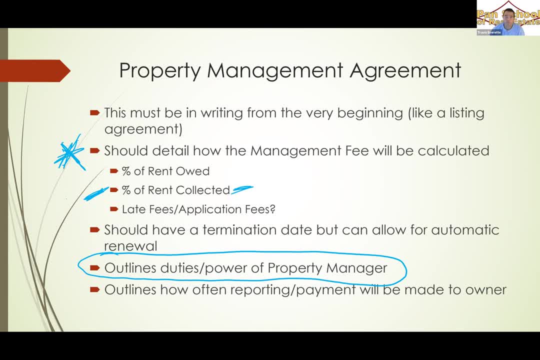 stating is: how often do we have to give financial reports to the owner? How often do they want to see the financial performance of the property? Some owners only want to see it yearly, Some want to see it monthly, Some want to see it every. 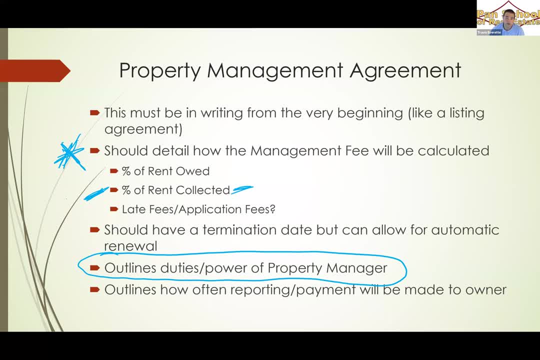 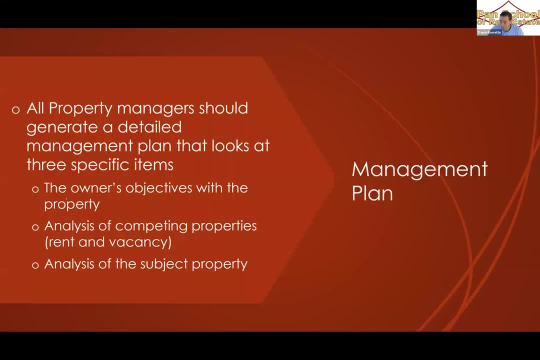 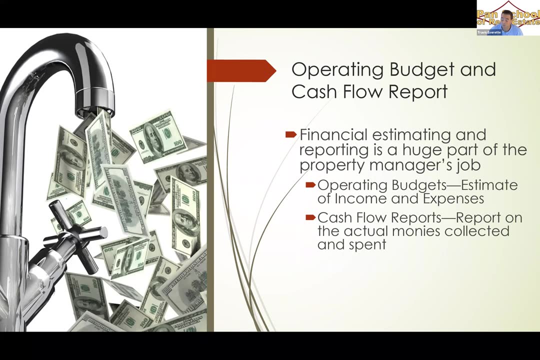 quarter. So it's really up to the owner how they want to see their financial reporting. I'm going to skip over this slide because you don't need to worry about that. You need to know the difference between something called an operating budget and a cash flow report. 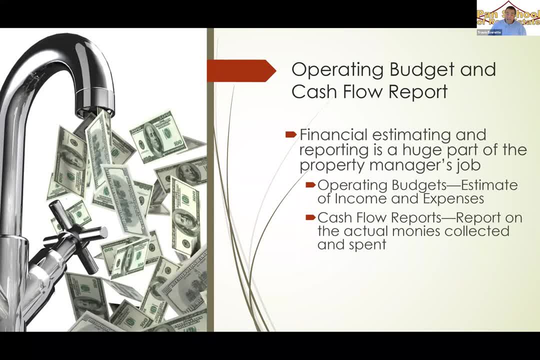 Here's what I will tell you. They are exactly the same thing, except they're called two different things based on when they're done As a report. they're exactly the same thing. An operating budget is a prediction of what you think the revenue and expenses will be. What do you think the cash flow? 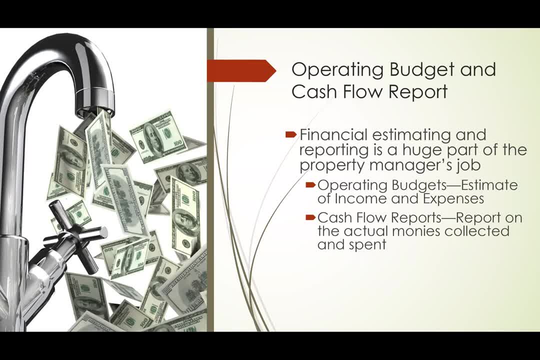 report is How much was actually spent, How much it actually was Exactly. So the operating budget would be something that you would give to the property owner in advance and say: this is what I think next year will look like The cash flow report would. 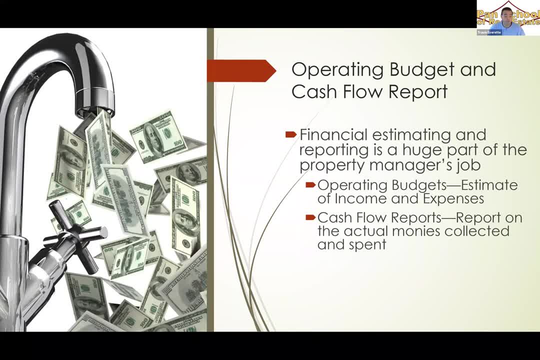 be a report that you would give at the end of the year to say: this is what the year actually was. That's the only difference between the two, But the reports and the math look exactly the same. Now I will tell you. 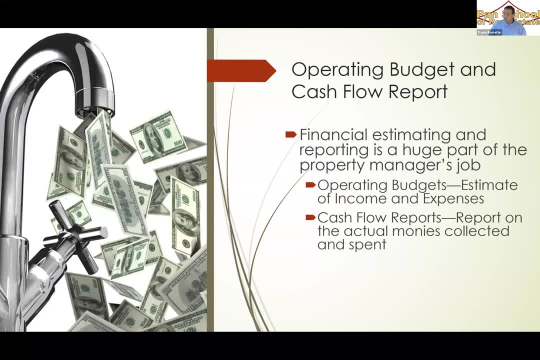 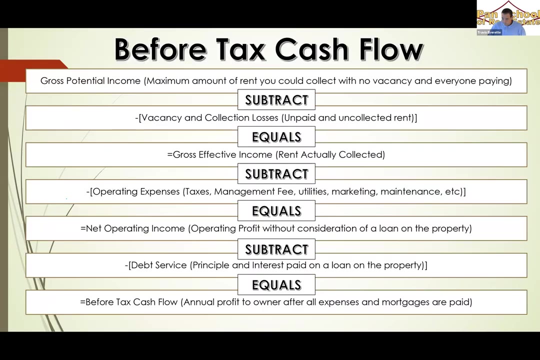 one of the greatest things they ever did for you all in this class is eliminated you having to do the math of a cash flow report, So you don't actually have to calculate cash flow, which you used to have to do. But that is a double-edged sword, because what they do 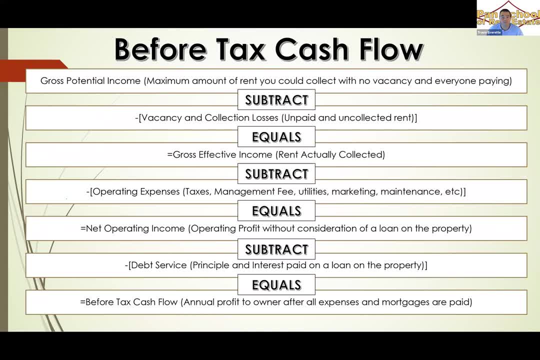 expect you to still know is the formula for calculating cash flow. They expect you to know how to calculate it, even if they're not going to give you a math question for it. And this is the formula for calculating before-tax cash flow, or just cash flow. Does it look complex here? 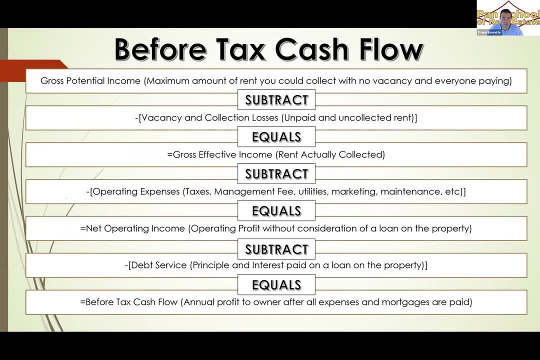 Pretty at all Long lot It went on there, right? Yes, Would you like an easier way to help you remember this formula? Absolutely, Of course. You don't have this next slide in your slide package, So I did put it on the OneDrive, It's. 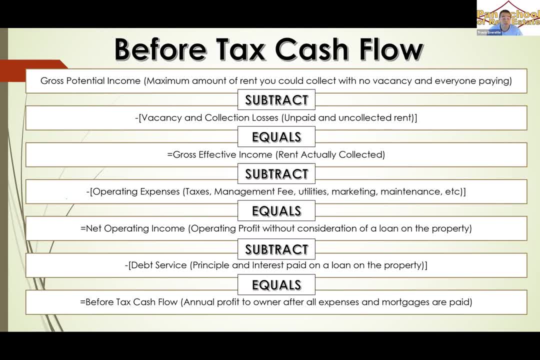 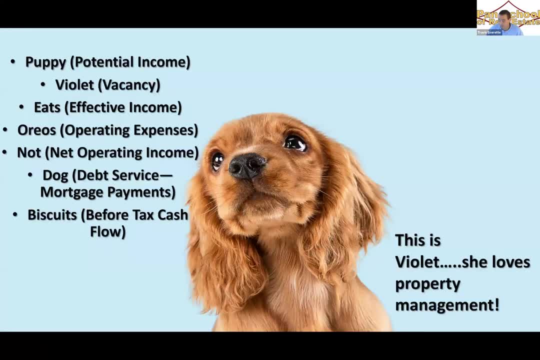 in the math worksheets folder on the OneDrive, but you could also take a picture of it or something if you wanted to. when I go to this next slide, because you don't have? Yes, So I did put it in the points here. 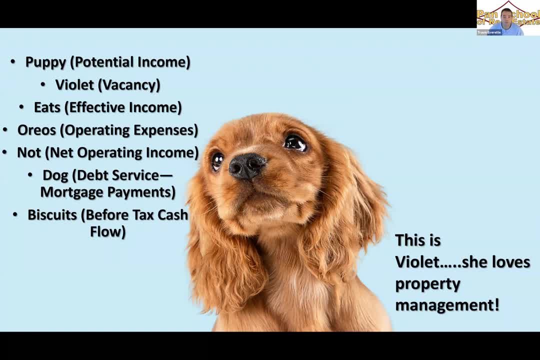 I pulled out the slides. if you're the first person who came to this, okay, We're going to start with this. before-tax order. I'm going to take this. I'm going to annoying the PowerPoint file. I'm going to write it down. 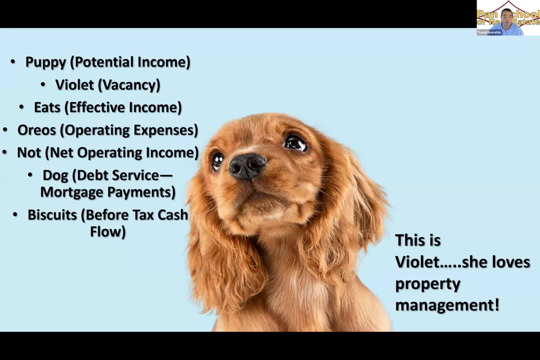 Just write it down now. This is keep me safe, Of course. By the way, if you're just starting out on youtube, take a second. not dog biscuits, i don't blame you. i like oreos a lot better too, and here's what that refers to. 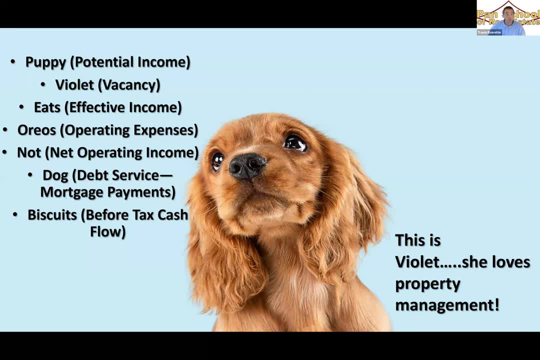 the p in puppy stands for potential income, the v stands for vacancy, the e stands for effective income, the o stands for operating expenses, um, the n and not stands for net operating income, the d for debt service, which is the mortgage payment, and then the b for before tax cash flow. 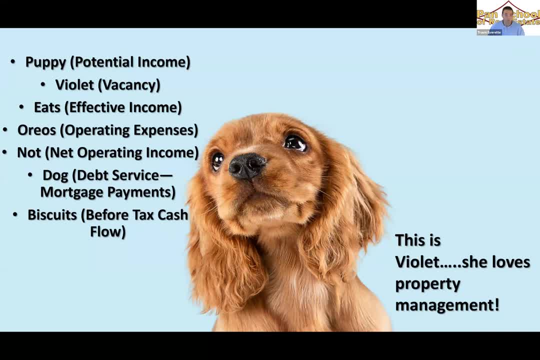 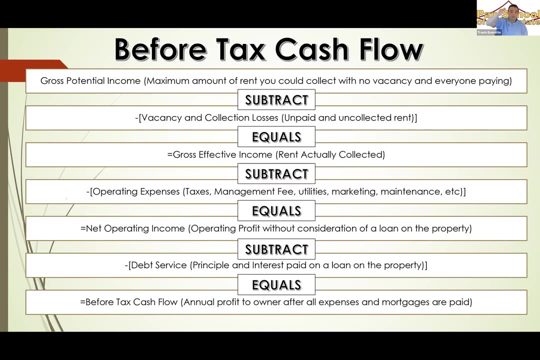 okay, so puppy violet eats oreos, not dog biscuits. that will help you keep this formula in order. now i'm going to back up a slide here. the good thing about this formula is it's just: this number minus this number equals this number minus this number equals. 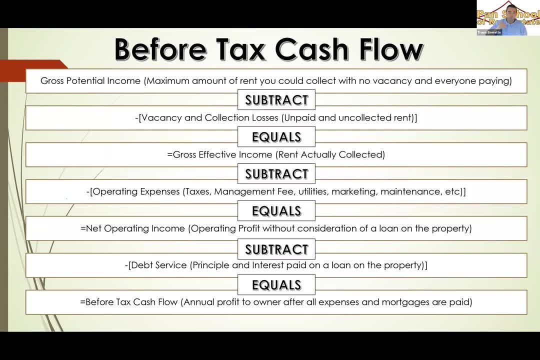 this number. it's always alternate: subtract equals, subtract equals, subtract equals. so if you look at the formula, it starts with potential income. so that's where the p comes in right. so puppy potential. so here's what potential income is. it's the maximum income we could collect if all the properties that we were managing for this person were occupied, and 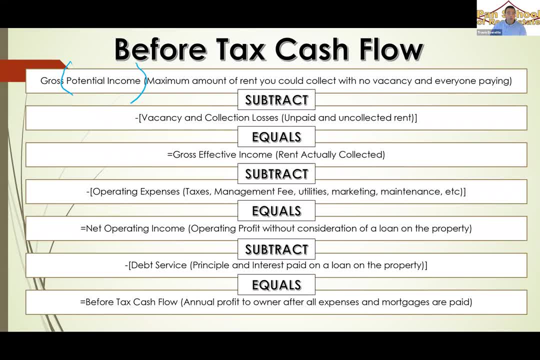 every tenant was paying their rent on time. as a property manager, we also call that fantasy land, because it never works out that way. you always have somebody who's either not paying or not paying on time. does that make sense for everybody? but we're not going to worry about those people. 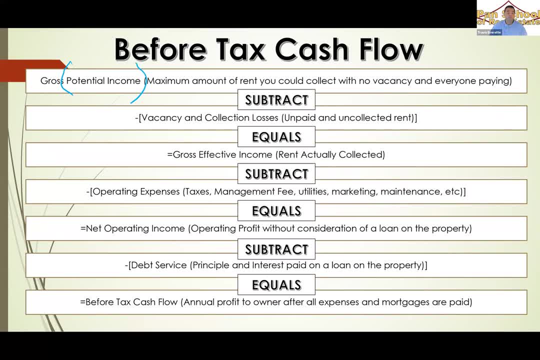 who are not paying on, not paying on time, because this is potential income, it's what we could potentially produce and that's our starting point and that's why everything's minus, because we're going to start going down from here. this is the most we could hope to produce and it's going to 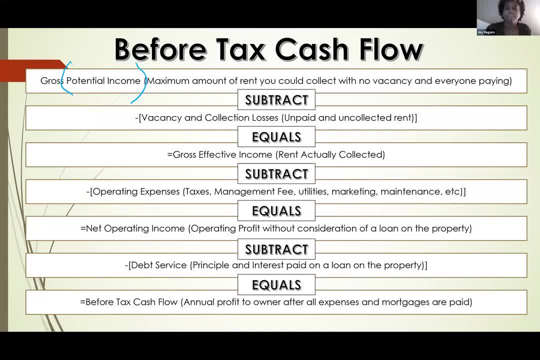 go backwards from here, you with me so far. so it's potential income and then minus vacancy. so there's your b vacancy. vacancy just means rent that you did not collect for any reason. either the units were vacant or there were people in the units, but they were not. what 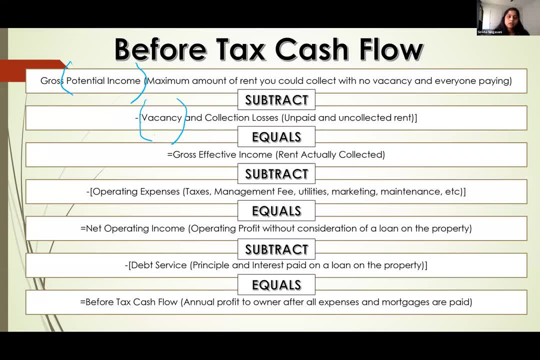 exactly so that encompasses your vacancy. gross potential income minus vacancy equals gross effective income or just effective income. effective income is the rent that was actually collected by the property manager, but we have to pay our expenses. so we're subtracting again minus our operating expenses, and we 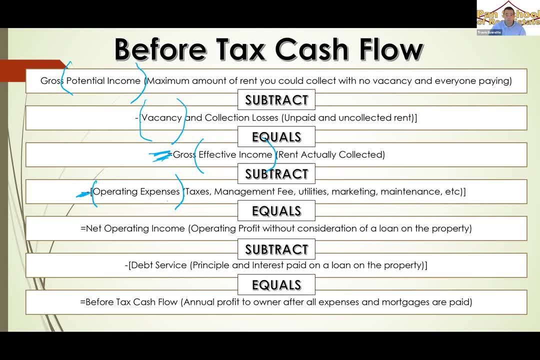 talked about what those were. that's pretty much every expense the property manager pays, with the exception of which one: mortgage or operating. it's good, very good, okay. so we're subtracting all our operating expenses and then that brings us down to this number right here: Net operating income. Net operating income is the amount of money that 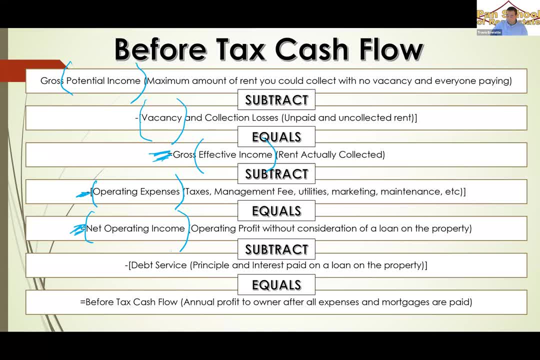 we produced by managing that property before we paid any mortgage notes that were outstanding. There's only one thing left to pay. What do you think that is A mortgage, A mortgage And what's another word for mortgage, Debt service? So we subtract the debt service and that equals our before tax cash flow. So this 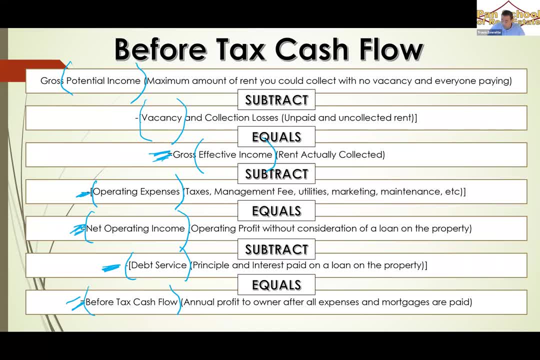 is before. So this is the spendable money. Another way you can say that is: this is cash to the owner. That's what the landlord gets to keep. That's what the landlord gets to keep. That's what. So at the end of the year, after we manage the property, this is the check we send. 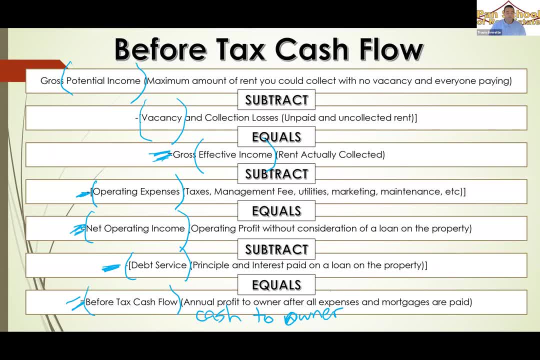 to the landlord. We send all these other payments to everybody else. We pay the maintenance, We pay the expenses, We pay the mortgage, We pay everybody else that's been paid. Here's your check at the end of the year, Mr or Mrs Landlord. There's your before tax cash flow And the reason it's called before. 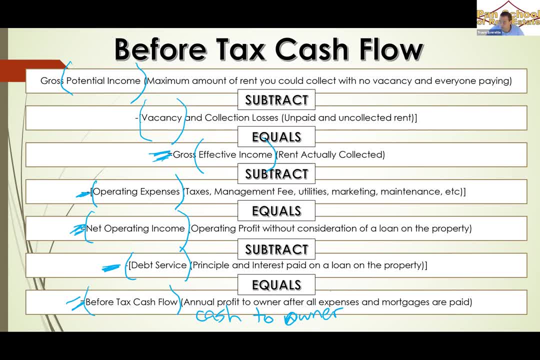 tax cash flow, because sometimes you will get confused and they say: well, wait a minute, taxes, These are the real estate taxes up here. What taxes do you think we're talking about down here at the bottom, Before the owner Taxes Income? These are before the owner pays income taxes And we don't worry about that as the property 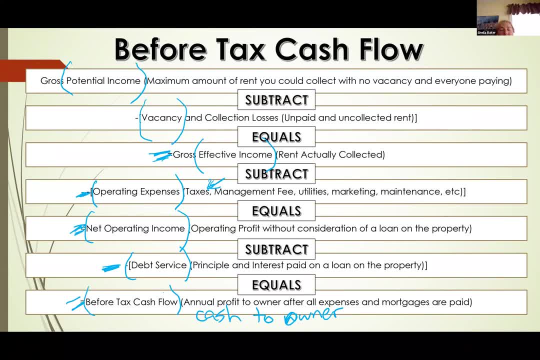 manager. That's for them to figure out. What might the question on the test look like? The question on the test will be some variation on the formula. It'll say you know what would be the which of the following is the best way for a property manager to calculate a? 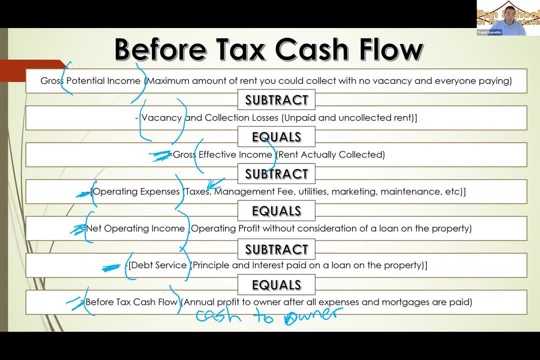 property's net operating income And you'll have to be able to calculate the net operating income And you'll have to be able to get the one that puts these in the correct order And we can't just spell out the puppy violet thing. 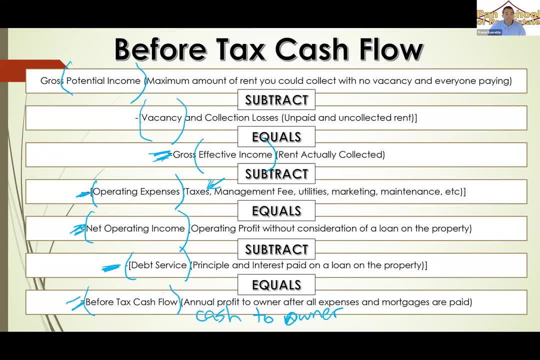 Well, you can, You can, I'm going to help you stuff out. for sure, I have a question, Go ahead. So obviously it's going to be multiple choice. So all you have to do is basically memorize the puppy violet little thing phrase you have And then just it'll have the 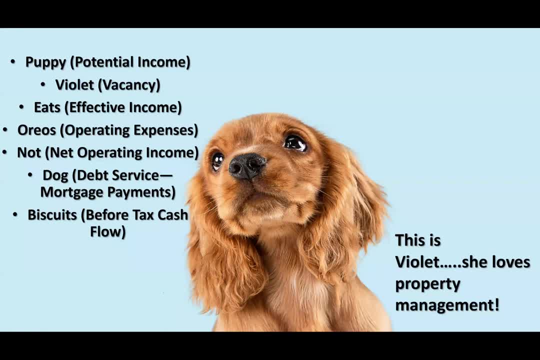 names on the multiple choice And then you can just spell out the puppy violet thing And then you can tell it what choice says That's exactly right. Oh, Doesn't that fit That? Okay, You don't have to actually know how to work with the math, You just have to be able to deal with the 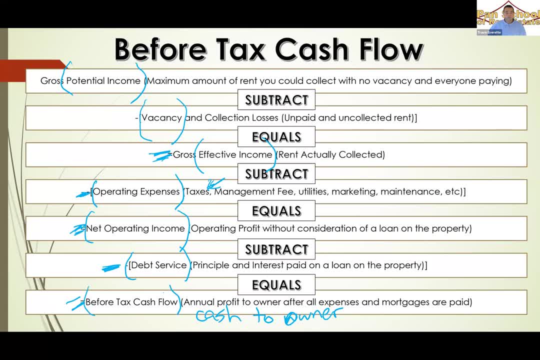 formula. So if they said to you which of the following- incredibly wasn't- your used to calculate net operating income, And one of the answer choices was: you take the gross potential income And you subtract the operating income from that number and you subtract the operating income from that number. 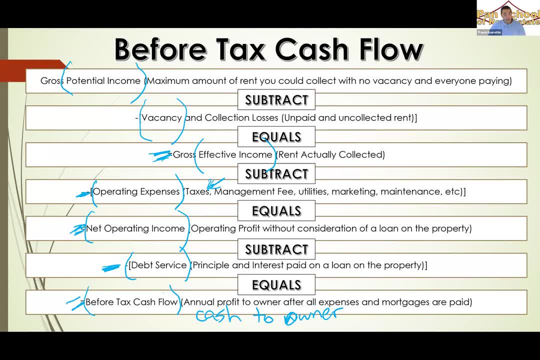 And you subtract the operating income and the debt service. would that be the right answer for net operating income or would that be too many things to subtract Too many? That'd be too many right, Because net operating income is before you subtract the debt service. So that's the kind of question you're going to get from. 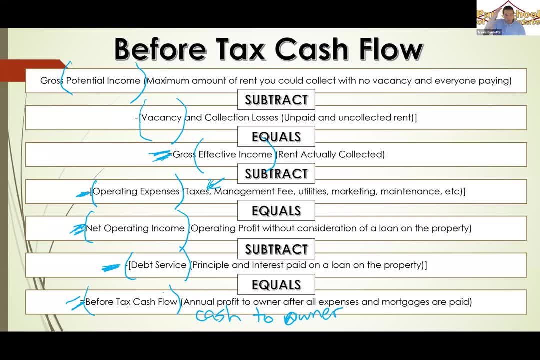 this. This can't just. do you know this formula? Do you know this progression of things? Could you say: gross potential income minus gross effective income equals the operating. No, that doesn't work. You have to go through the steps. You have to go through the steps. Yeah, you have to go. 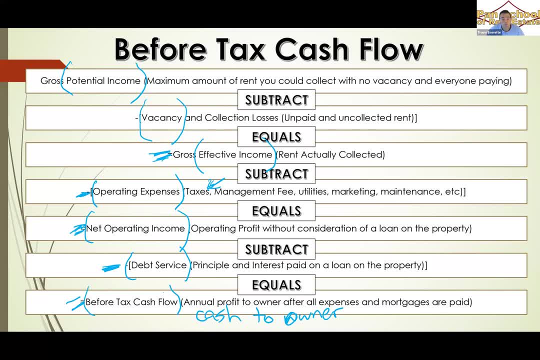 through the steps. I have a question for you. Okay, So whenever, like I was looking at this and reading it, I understand this, but then I was thinking about how, like we do things at the real estate office And like, whenever we bill out or we give our owners their statement, each month it has our property management fee, which the least amount that we will do is $100 for a property, And then so- or at least my chart, I'm sorry- And then the rest of the time they get, the remainder of what their rent will be So like if the rent is like $1,100,. 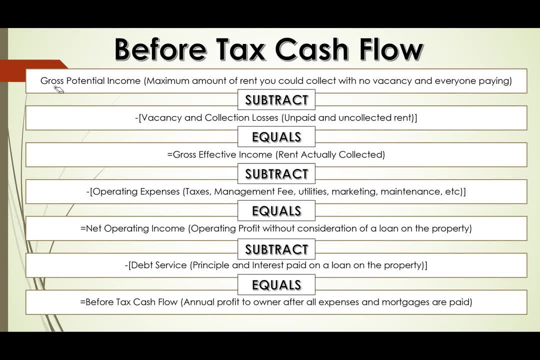 we take out $100 for our management fee and then the owner gets that $1,000, and they're responsible for, you know, making their Other payments, Yeah, their other payments, and stuff like that. What I will tell you is that when you get into bigger volume property management, 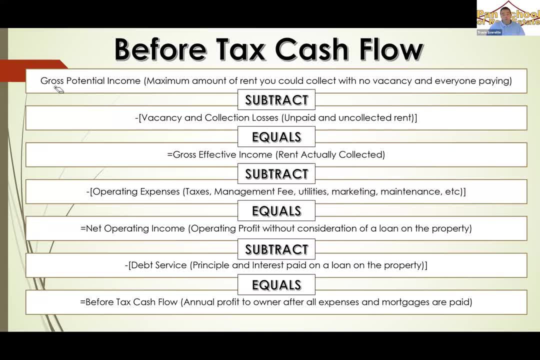 where you're managing, you know, 100 units for one owner. they would expect their property manager to do all of that. They don't want to pay the property taxes, They don't want to pay everything, pay the insurance, they don't. they just say send me a check at the end. okay, and so like, right it. 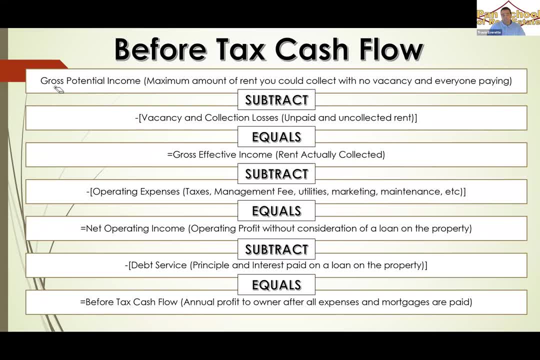 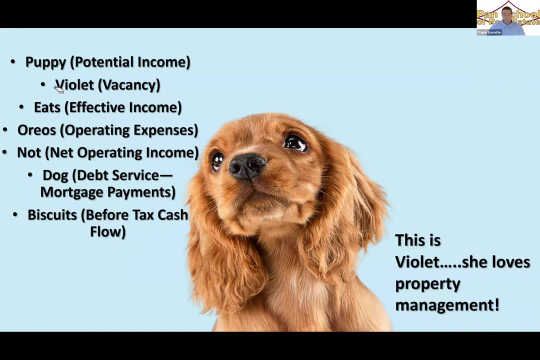 does depend on what type of property management agreement you have. okay, because i know, like we have a, a gentleman who is local who literally buys hundreds of properties and he splits it into his kids name to build a college fund for them, yeah, and so like we manage all of those. 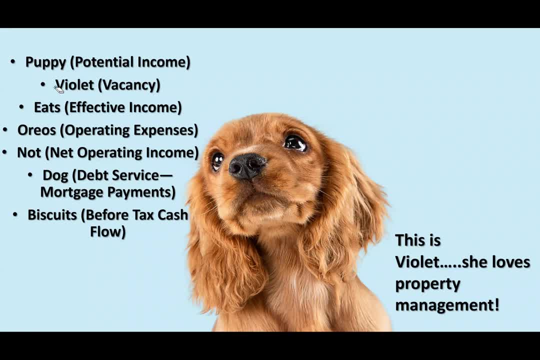 properties, but they're in each of his kids names and then he's got some in his wife's name and then some in his name. i'm really surprised he hasn't asked how to take over managing the entire cash flow, because that's usually what those i think he probably is, but he just went and got his real. 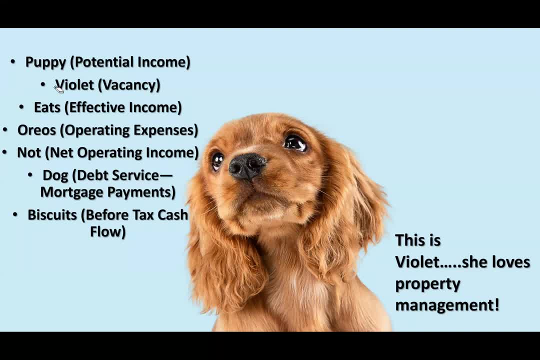 estate license, so i don't know if he's planning on taking over it or what, but i just didn't know. if we would, you wouldn't even do that same like equation with something like that where you're not having to take care of well, you adjusted version of it, you and, and they would. 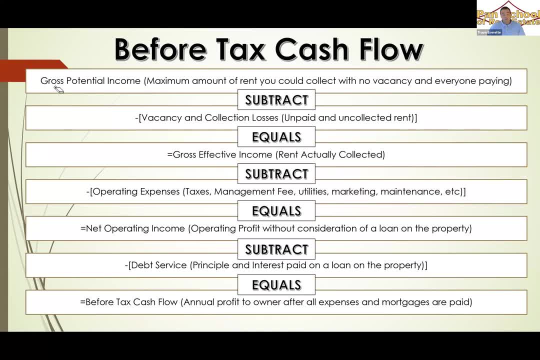 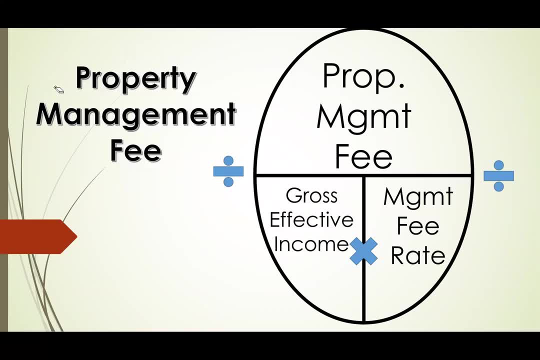 understand they still have expenses to pay once they get the money, but this is how they, this is how the ultimate accounting gets done. okay, gotcha, okay, all right. how do we calculate a management fee itself? well, that's just going to be the gross effective income, which, remember, we said gross. 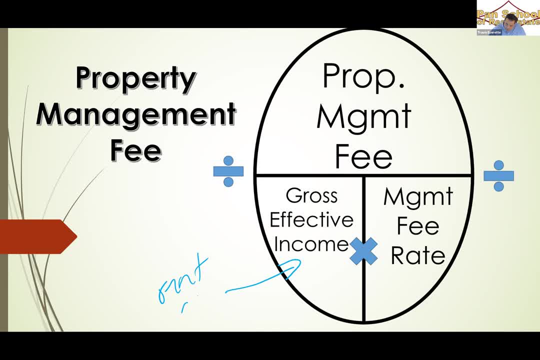 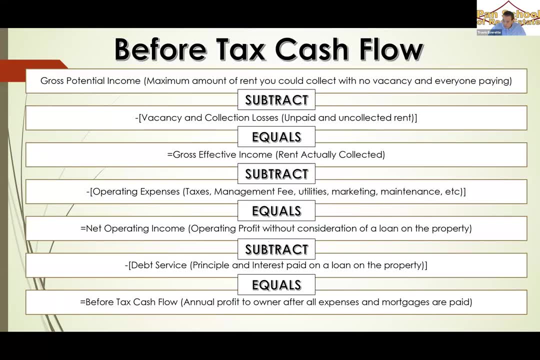 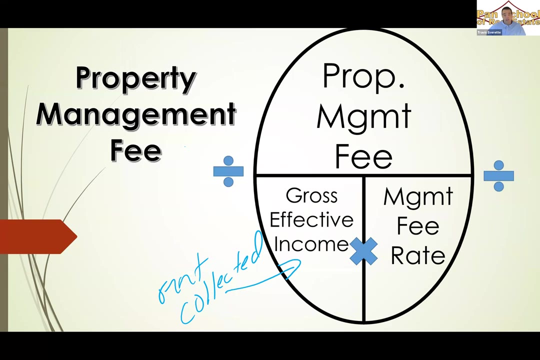 income is the same thing as rent collected, because if you go back here you look at gross effective income, it says that you take the gross potential and you subtract the vacancy and that equals gross effective. that's why it's rent actually collected. so to calculate the management fee, if you were doing that math it would be the 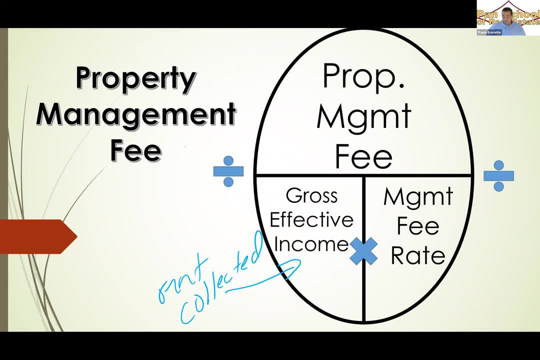 gross effective income or rent actually collected times, whatever the rate is um. so you know a lot of property managers say: well, how do you calculate that? so that's just going to be the gross effective charged. maybe a 10% rate, 10% of rent actually collected becomes the management fee. 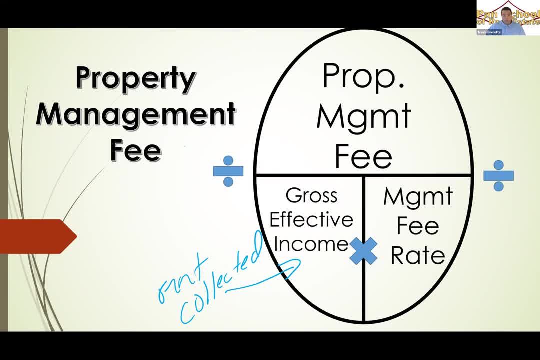 And that's how you calculate a management fee. Again, probably not math. they would ask you to do anymore Math. they used to ask you to do but math they would not ask you to do now. But you need to know the formula for it in case they throw it out there as a test question. 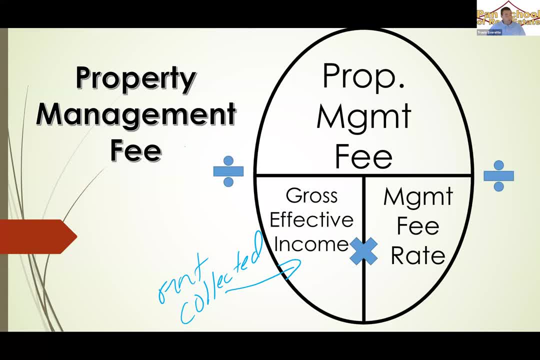 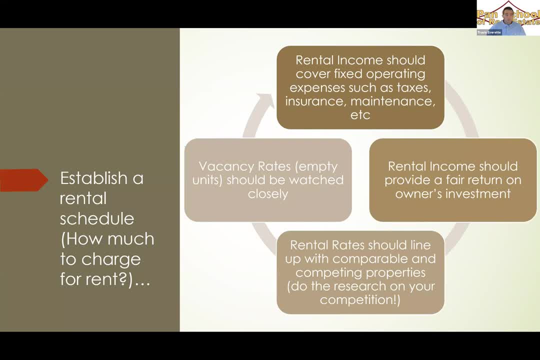 of how you calculate a property management fee. Well, it's the rent actually collected or gross effective income times the rate. How do property managers decide how much to charge? Can you go back one slide? Sure, I'm sorry. So it's gross effective income times the rate. 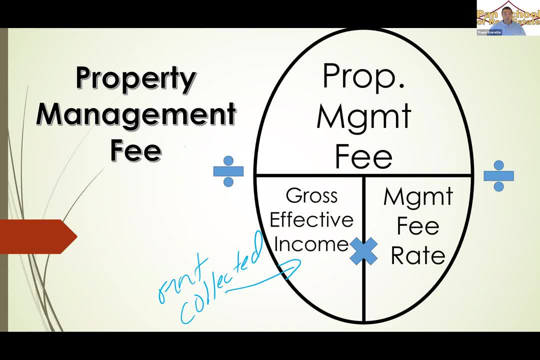 Correct. So you would be paid a percentage of the rent you actually collect as the property, Yep, Yep, And that equals the Potential income. No, sorry, property management fee. That's the property management fee. That is correct. So like, for example, if I am managing, 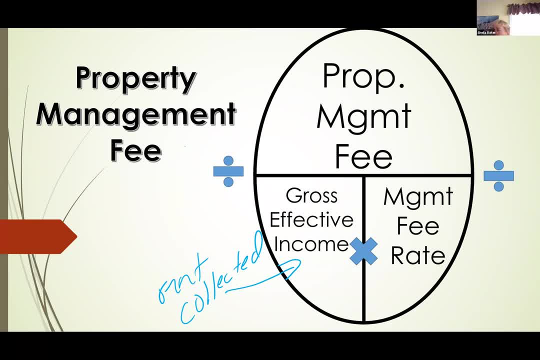 an apartment complex and I'm charging a 10% management fee and the gross effective income for the month is $100,000, that's the rent I actually collected for the month and my management fee for the month would be $10,000. 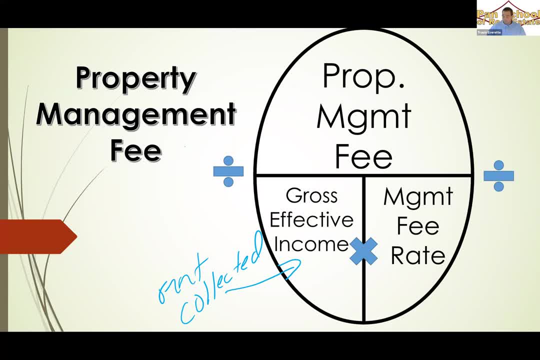 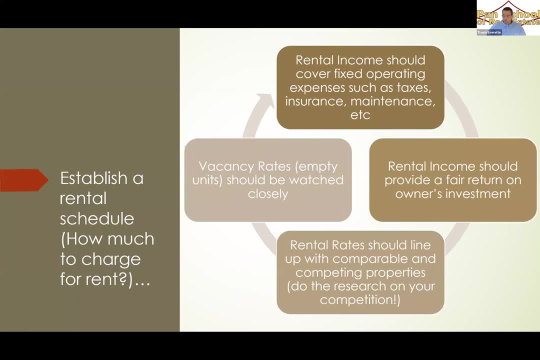 If I was charging a 10% Right. You may see test questions and I told you this chapter would be very short. There's not many potential test questions. quite honestly, they would ask you from this chapter. but you may see test questions about how property managers go about establishing the amount. 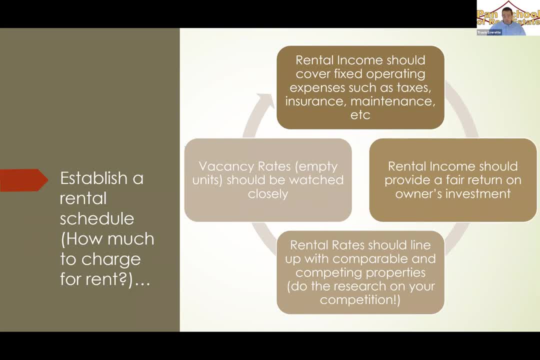 of rent that they should charge to tenants in a particular property and what would impact that? And there are a lot of things that impact it. However, I want to rank them for you as far as importance, in case they ask something like that on the test, Like what if they ask you? 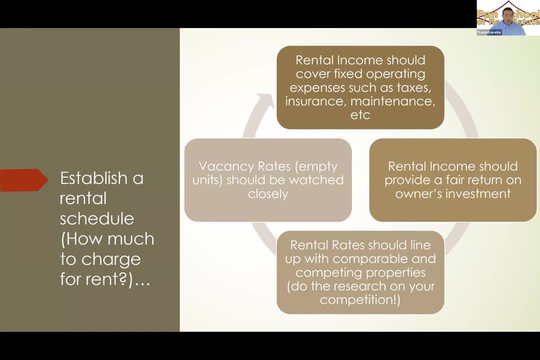 what's the number one thing that a property manager should look at when setting their rental rates? This is number one, right here. So number one: you're going to see what others are charging in the area, what the competition looks like. That's going to be the most important factor in determining how much you charge as a property manager. 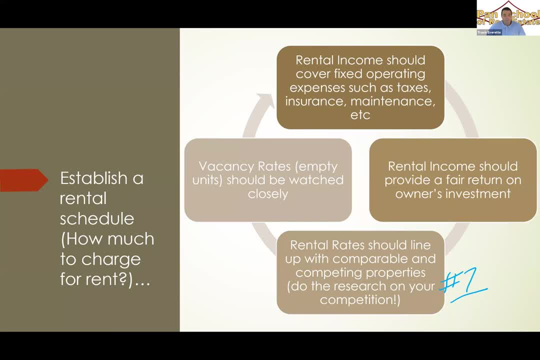 rent and, if you think about it, that just makes sense because you're in competition with those surrounding properties. you're competing for the same tenants. So that's going to be the biggest determining factor of what you can charge for rent. What's the second most important factor in determining how much we charge as a property manager? rent? 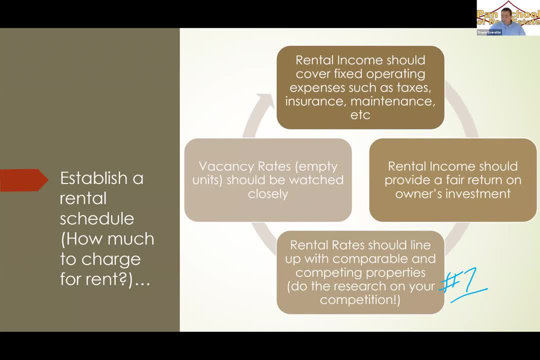 You're competing for the same tenant, So that's going to be the biggest determining factor of what you can charge for rent. What numbers to avoid? 13., 16., 17., 18.. other things that impact it are vacancy rates. you know, are we paying for our? 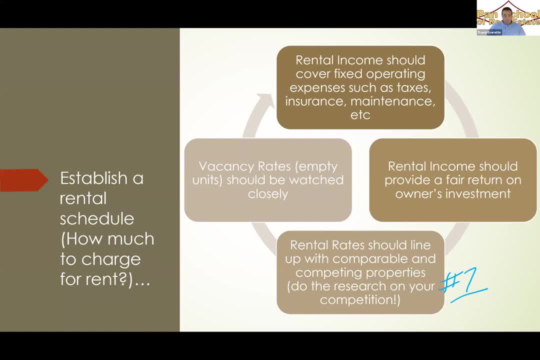 expenses, all of those things, but definitely number one biggest factor is going to be: what is, what are the prevailing rates in your area? what are other properties that you're competing with charging? so if they ask you to sort of rank that on a test, I would say that be number one as far as dictating what 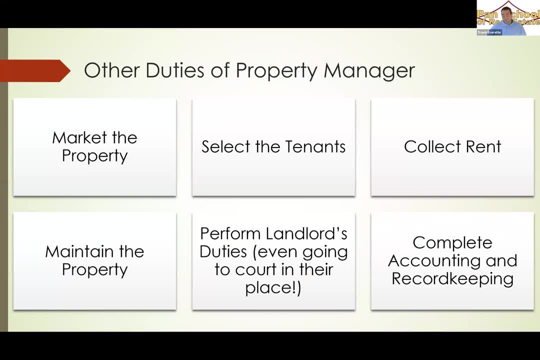 you charge some things. the other things they like to ask you on the test are: what are the responsibilities of the property manager and what are not the responsibilities of the property manager? all of these things would be expectations of property managers for most properties market the property. so 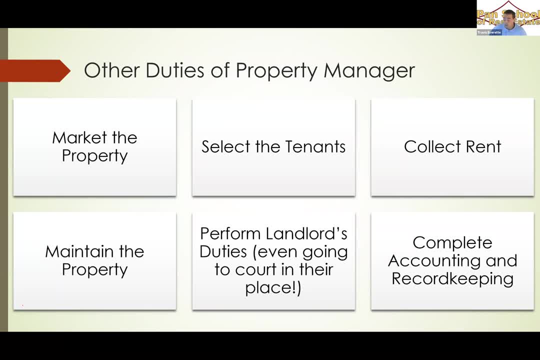 find tenants. that's, you know, huge part of the job: choosing the tenants. so taking the applications, looking through the applications, deciding which tenants to accept, which tenants to reject- that would be a big part of the property managers job. collection of rent: as far as owner's concern, this is probably the biggest part of a property managers job. 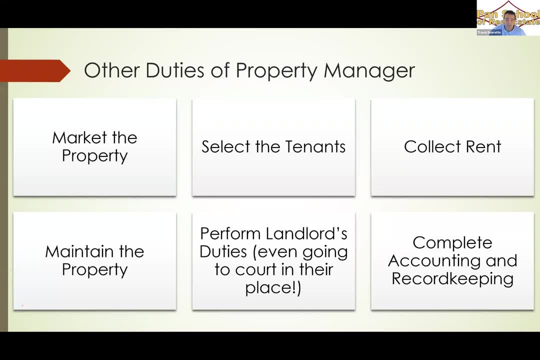 because most owners who hire property managers have tried to do it themselves before and they found themselves struggling to collect rent and that's why they hired a property. they want us to be the bad guy. that's why you should never getting into property management. um, with a soft heart, i worry about britney. she's not gonna make. 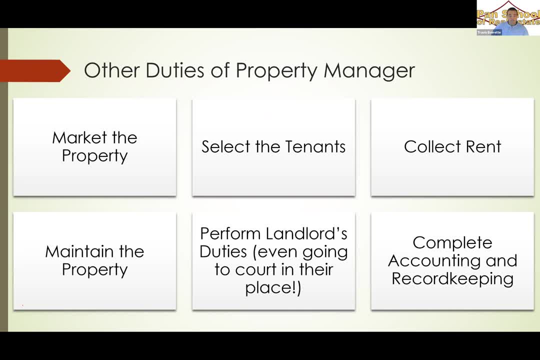 it. she's too nice in property management. um, you gotta. you gotta be mean, being that, you just gotta be not kidding. you don't have to be mean, be a property manager, but i just like, i just want everything to be fair and i can't like, i don't know, it's just every scenario that we've 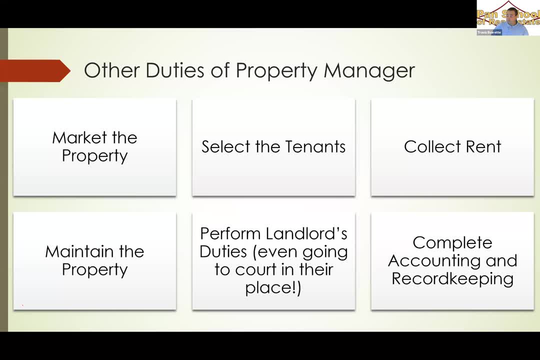 done. i got out of it. i laugh about it, but i'm i was up to i was too much of a target i was. you know, i just had sucker written across my head. i mean people could cry and i just like, oh, don't cry. and then i and they got over on me so i just had to get out of it. i had one tenant, her, her. 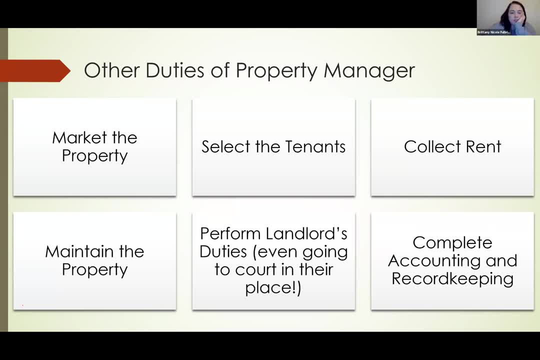 mother passed away while she lived in the property, and then i realized about halfway through the conversation that this was the third time her mother had passed away. see, that was the kind of stuff i dealt with when i was a property manager. so, um yeah, it was not a good fit for me. it was not a good fit for me. 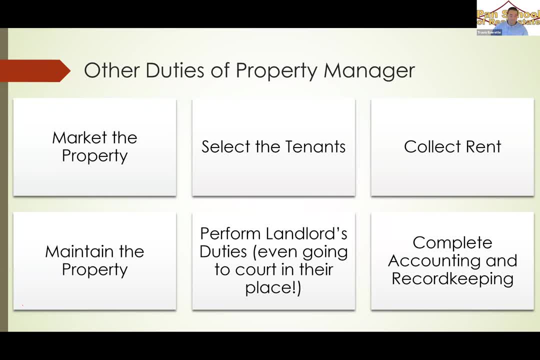 so i had. i had a lady that i worked with, an older agent and she said, honey, here's how you know if you're suited for residential property management. if you can kick a single mother with three kids out on christmas day, you're well suited to be a property manager. if not, you ain't suited for. 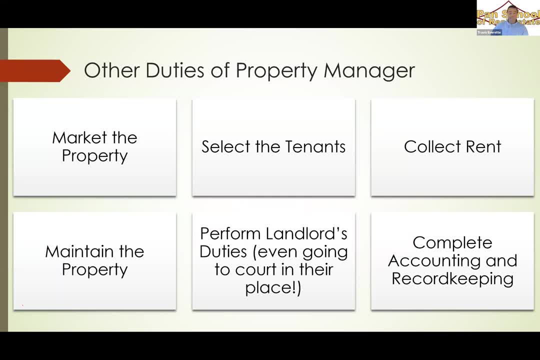 that business. that's what she told me, and i was like, oh gosh, okay, um. it is a business that hardens you, though, because it was a lot of stuff you deal with as a residential property manager, so it definitely changes your outlook on things, i think. sometimes. 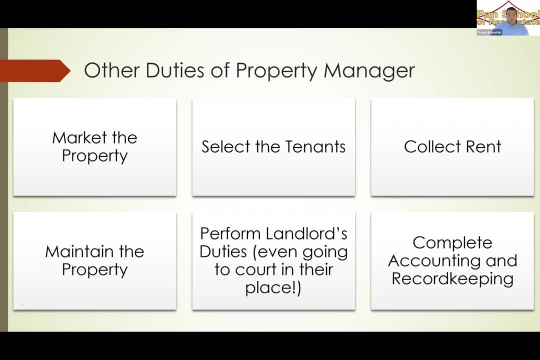 um maintaining the property- huge part of the property manager's job- um performing the landlord's duties, and that means, yes, even going to court in their place. so when there is, if you see a test question about eviction act, um, this is kind of one they might ask you about right here. you know who would go to court and 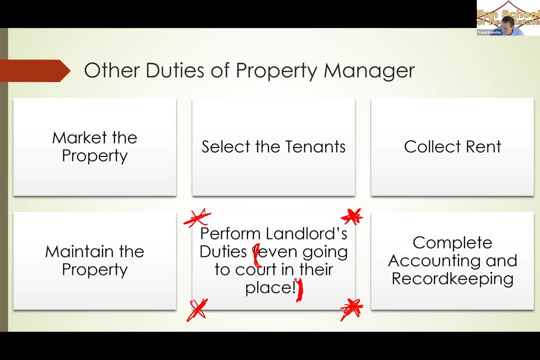 file for an eviction? who would testify? who would handle that court action? would it be the landlord? would it be the property manager? the answer is: it would be the property manager. that's one of the functions that they generally expect, um, of a property manager, um, and then, of course, provide. 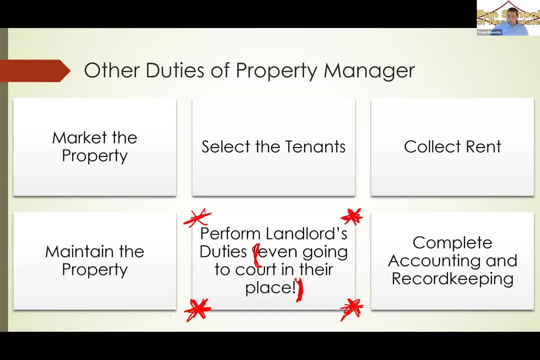 them with accounting for their money. those are all the functions of a property manager. now let me tell you what's not the function of a property manager. the kind of stuff i've seen pop up on tests that people fall victim to the the profit generated from the property. who does that belong to? does it belong to? 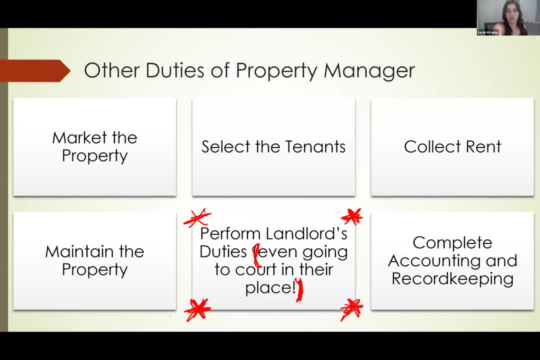 the property manager, does it belong to the owner, landlord- that's their money. don't- don't answer a test question- that the property manager gets to spend the the profits generated by the property or decide how to invest the profits, or anything like that. no, no, no, no. that's their money once we have managed the property and created that profit. 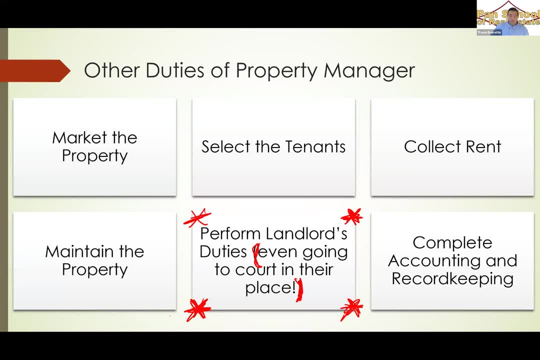 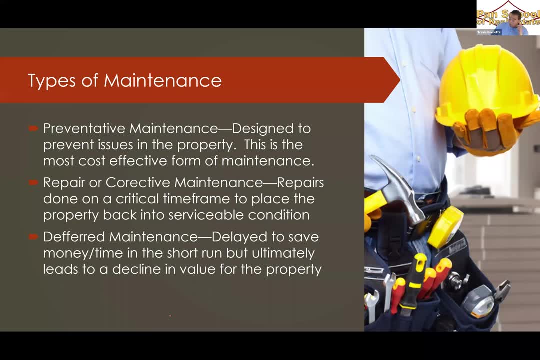 we send them a check and then they do whatever they want to do after that. okay, so be careful of that. um, be careful of that. some different types of maintenance you may be faced with on the test. um, uh, preventative versus corrective maintenance or repair. um, one is done before there's a problem, to prevent a problem. the other is done after the problem is. 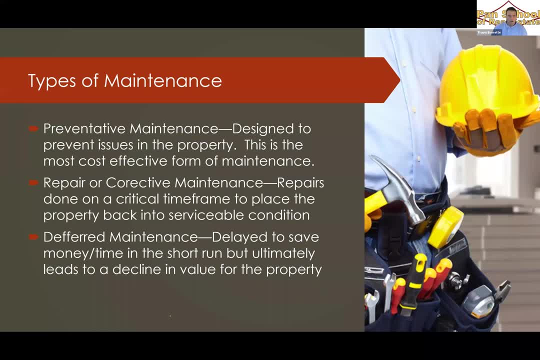 known to correct a problem. which one do you think is more cost effective, long term preventative maintenance or corrective maintenance- if you're a property manager, the biggest goals of a property manager is to- and most property managers actually keep two different um line items, one for preventative maintenance expenses and one for corrective maintenance expenses- because they 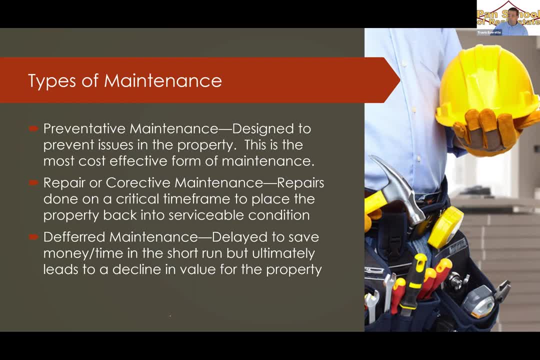 want to make sure that they're mostly doing preventative maintenance. so preventative maintenance would be things like going in and changing all the air filters on the hbac system. going in and making sure that, um the property is well insulated, you know, so you don't have burst pipes or that sort of thing, um pumping the septic tank out so it doesn't back up. 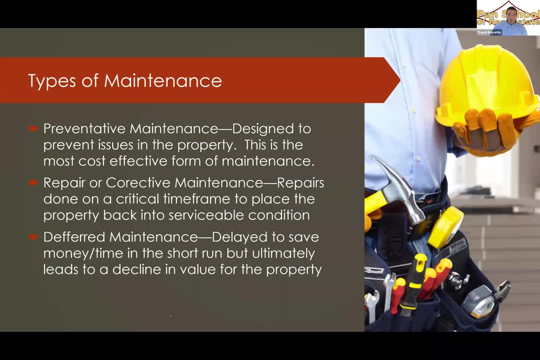 but doing it before it backs up, um, whereas corrective maintenance would be doing those kinds of things on an emergency basis because something's broken. corrective maintenance is really cost ineffective, primarily because you have to pay people more when they have to come out on the emergency basis. um, and so when you're you know if i can schedule um things. 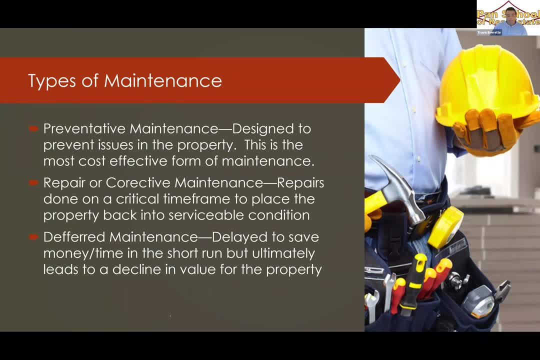 as preventative maintenance. i can get somebody to work all day and accomplish 15 tasks and pay them the same amount of money i might pay them for one emergency corrective visit. so um, preventative is much more cost effective for a, a property management. um deferred maintenance is the kind. 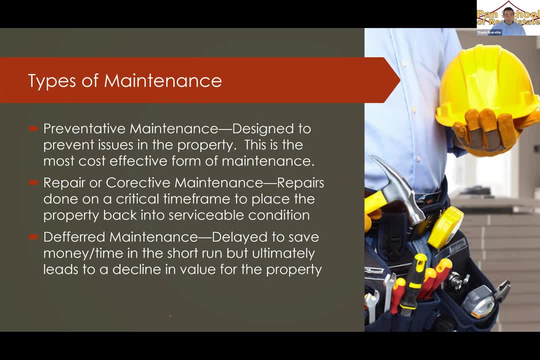 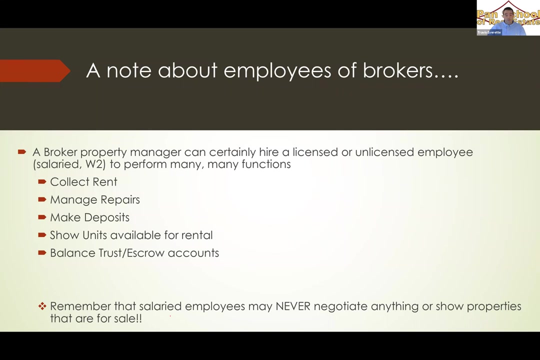 of maintenance we should avoid at all costs as a property manager, and that's maintenance that's never done, it's put off. deferred means delayed until a later date, because deferred maintenance almost always leads to leads to more corrective maintenance. so just make sure you can differentiate on the test. um, we've already talked about the exemption for employees uh w-2 salaried employees. 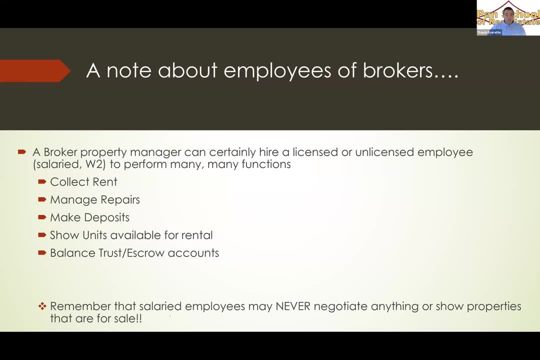 of both the property owner and of the real estate broker being exemptions to the licensing rule. don't forget that. that rule from way back in the beginning. who needs a real estate license? well, generally speaking, somebody who's doing any kind of a real estate activity and they're doing the service for somebody other than 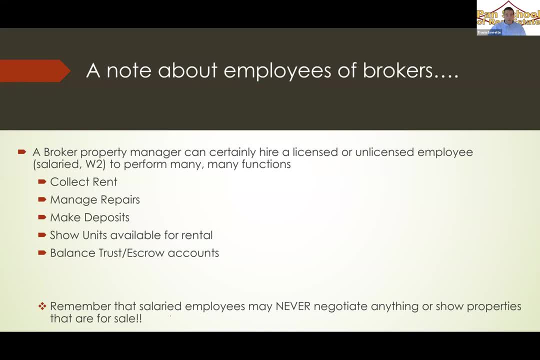 themselves and they're being paid for it. if they're doing all three of those at once meet the license. but there are a couple of exemptions for that and one of those is the salary w-2 employee of the property owner and another is the salaried w-2 employee of a real estate broker. 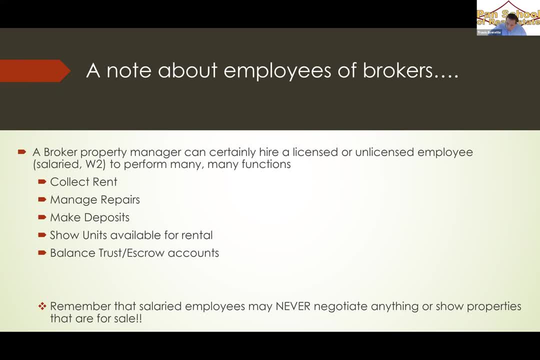 so you're probably going to see test questions. i would say this right here: for sure is going to show up as a test question in the north carolina section of the exam something related to what can a salaried employee of a real estate broker do? and they can do a lot of things. they. 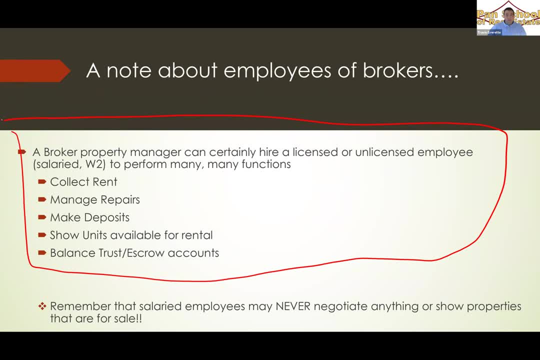 especially when it comes to property management. they can collect rent, they can schedule showings, they can manage repairs, they can make deposits, they can show rental units that are available. they can balance the trust account. now it's going to be the broker in charge who's responsible for the trust account, but they can balance it. they can be the bookkeeper, they can. 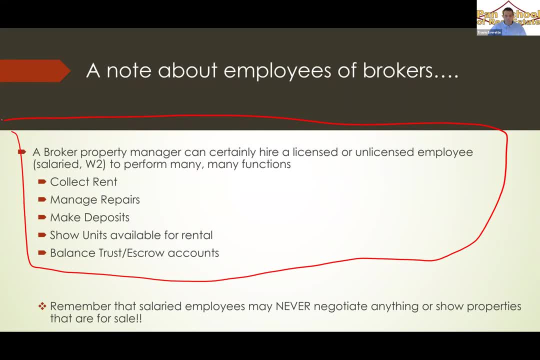 deposit money. they can do all of that stuff as an unlicensed assistant. they can place advertisements as long as they don't create the advertisement. it has to be the broker who employs them who creates advertisement. they can put stuff in the mls as long as they get the information from the broker. 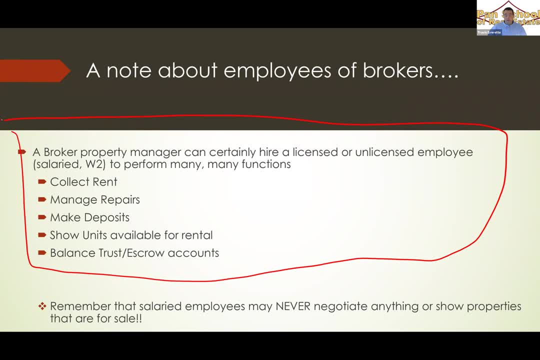 that's allowed. but the salaried employees of real estate brokers cannot do two things ever. they cannot negotiate in any way, or they cannot stand, or they cannot show properties that are for what sale? for sale stuff that's for sale. so if you got a test question, it said cassie is the salaried employee of broker bob. 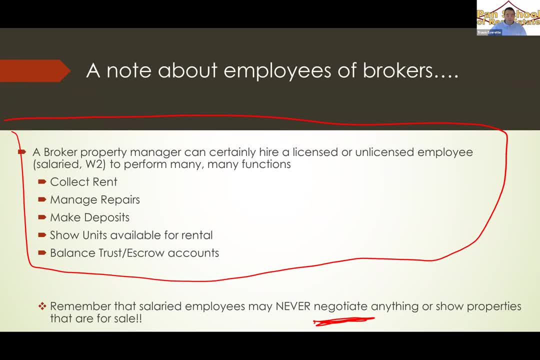 and bob is holding an open house on saturday, and asked cassie to hold the open house in his place. can she do this? what's the answer to that? no, no, because an open house means the property is for what sale and she cannot do that. she can assist bob if he's there, but she can't be there by herself. 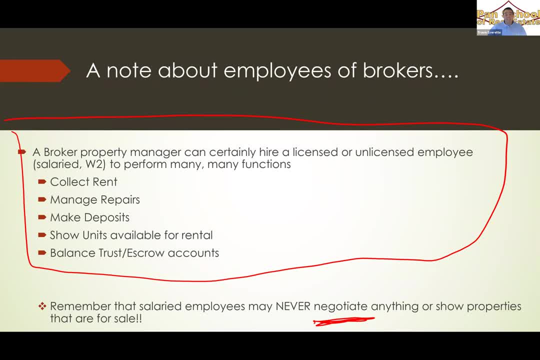 but could cassie show tenants rental properties that bob can't do? and this is so important because i think, at the very least, we won't be talking about anything that had to do with rent or for rent, and maybe not as much of what bob was managing that were. 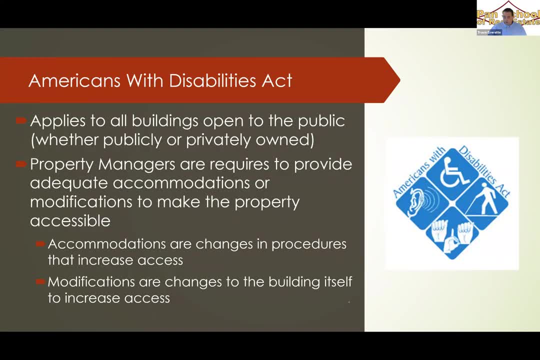 available for rent. yes, yes, yes, she could, she could, okay, so you probably see that kind of a question as well. um, i'm going to hold off on the americans with disabilities act for a long discussion, but i'm just going to mention it here. the ada, or americans with disabilities act, impacts property. 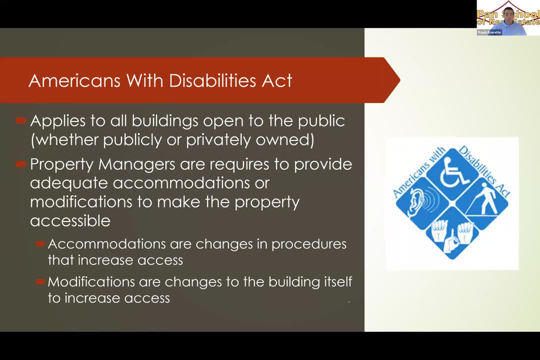 that if you are managing the commercial space, and so may as well just say commercial real estate- if you're managing a commercial piece of property- because, notice, it says buildings open to the public- you have to follow the Americans with Disabilities Act. the Americans with Disabilities Act requires: 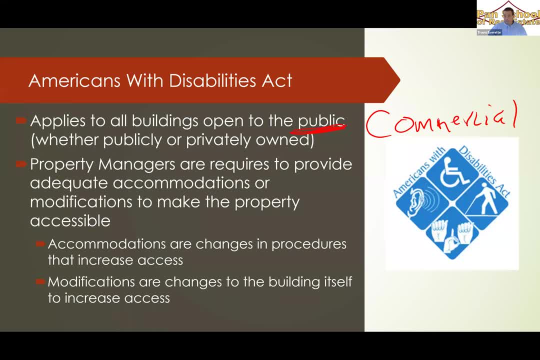 equal levels of access, regardless of physical handicap. and you can provide that access as a property manager in one of two ways: you can either make an accommodation for this person or you can make a modification for this person. it says here: an accommodation is a change in our procedures. 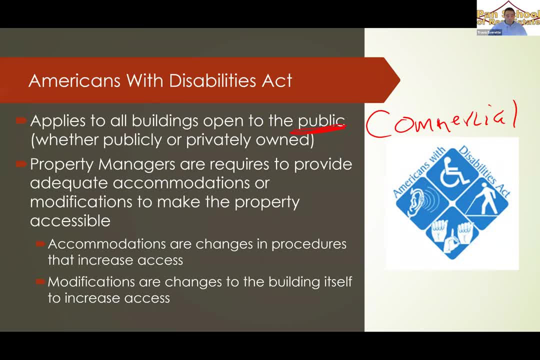 so I'll give an example. if I own a restaurant, I probably don't allow animals in the dining facility, but allowing a service animal would be an example of an accommodation I would make under the Americans with Disabilities Act. it doesn't require me to change anything about the property, it just changes my 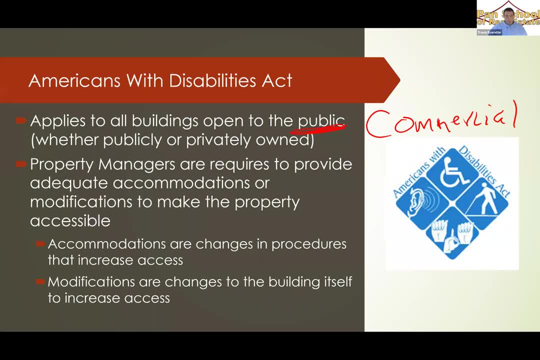 operating procedures. does that make sense for everyone? whereas a modification is an actual physical change to the property or structure itself. so if I installed a handicap accessible ramp, for example, because we didn't have an elevator, that would be a modification. if I were to put the handles in bathroom stalls, that would be a modification to the property, because 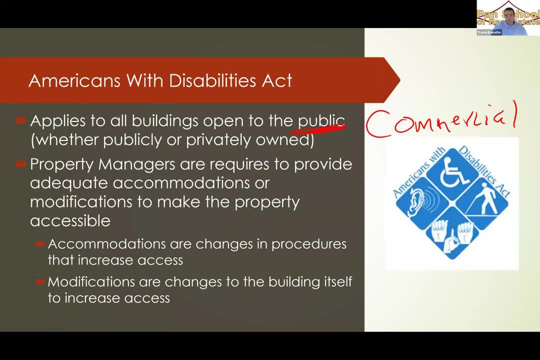 it's a physical change, so just make sure you know the difference between an accommodation and a modification and what the Americans with Disabilities Act says. if you're managing a public space commercial property, you have to be willing to make either an accommodation or a modification, whichever, in order to 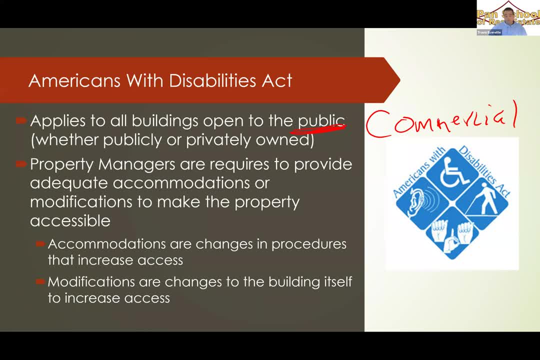 provide an equal level of access. sometimes that choice will be to make a modification to the property and sometimes it'll be to make an accommodation by changing your operating procedures. I use this as an example a lot when I teach this. in my hometown of Tarboro, the post office is this huge. 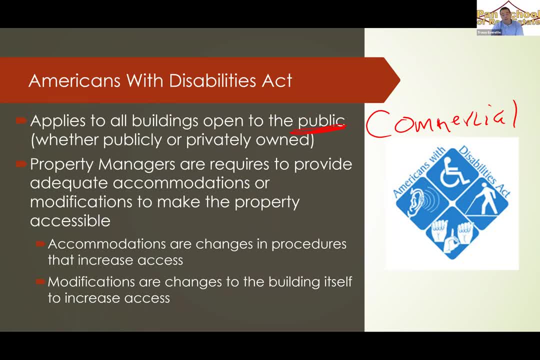 granite building on Main Street and you got to go up like 25 steps to get to it. huge staircase outside it goes up to it. the building was built in the early 1800s. there's no elevators in there, so does that present a problem for somebody who wants to go to check? 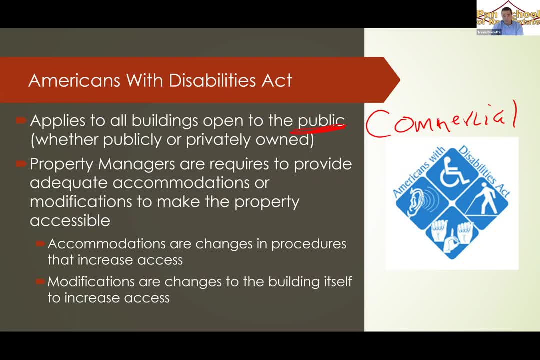 their post office box, if they are wheelchair back, for example, absolutely, and so they had to, because of the Americans with Disabilities Act, either make an accommodation or a modification, and they elected to go with an accommodation. they elected to say we would rather accommodate these people than change the building, because 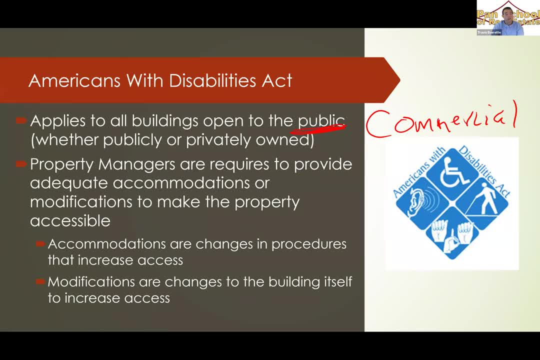 it would be so expensive, so cost prohibitive to change the building, and so here's their accommodation. there's a sign out front of the post office that says: if you have a disability access related need, please pull around to the rear. when you pull around to the rear, they have a parking spot. it's reserved. 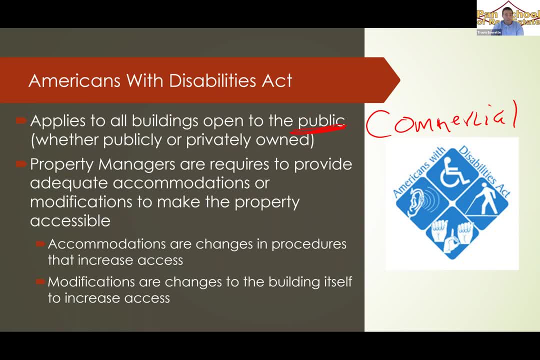 there for those with disability access needs and there's a buzzer that they press the button and it's the intercom. it calls somebody who's upstairs in the post office and you say I need this, I need to do that, and they bring whatever you need down to you and take whatever. 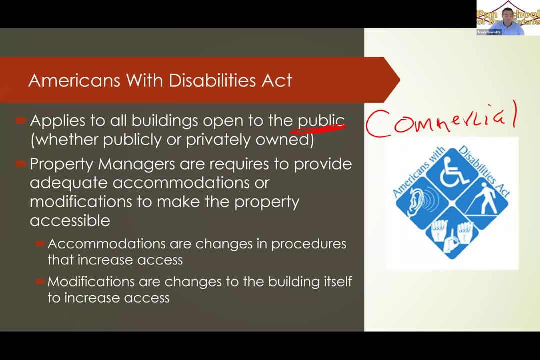 you need back up, and that's their accommodation versus modification. so the ADA does not specify which you have to do, it just says you have to do one or the other, and you see this in effect almost everywhere you go. how many of you? I'll tell you one thing. that was: 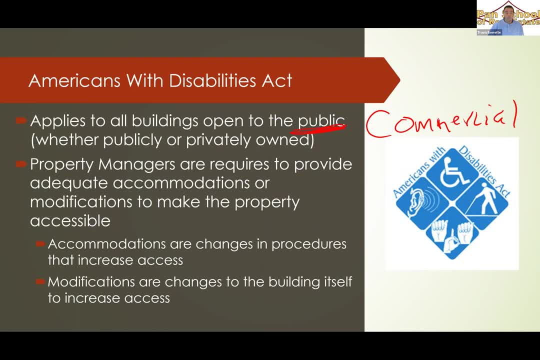 exempted from the ADA for a long time, until a few years ago. how many of you noticed a few years ago that swimming pools at hotels started to have something that they had not always had in the past: the chair. they have a chair and at one point in time, properties that were constructed before the ADA was in. 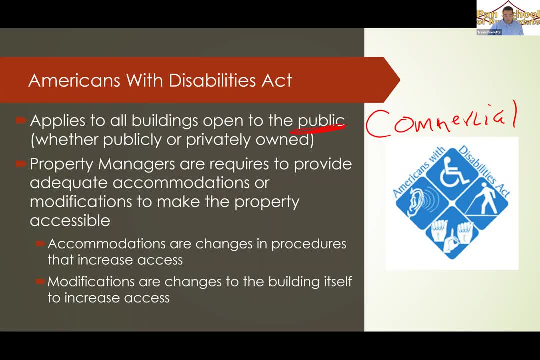 effect did not have to come into compliance. that has since been changed and now they have to come into compliance so proactively. so you see a lot of hotels either adding lift chairs to their swimming facilities or closing pools all together because that you know the cost of installing the chair. so 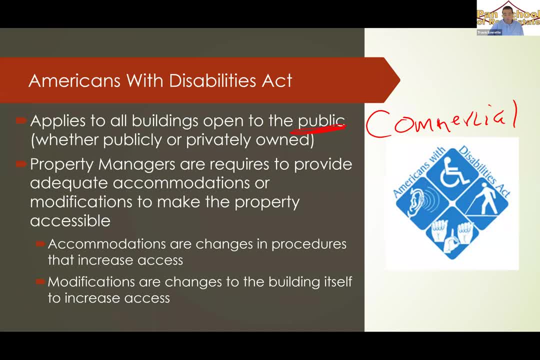 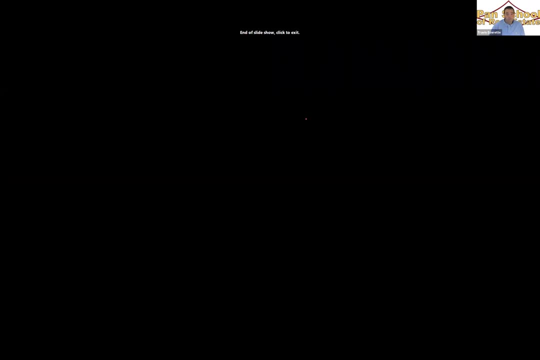 those are. you know how people respond to these. you know accommodations or modifications, so it's all about providing a the same level of access, and that is it for chapter 12.. Thank you, Yeah, Travis. I don't know a lot about property management, but it seemed like. 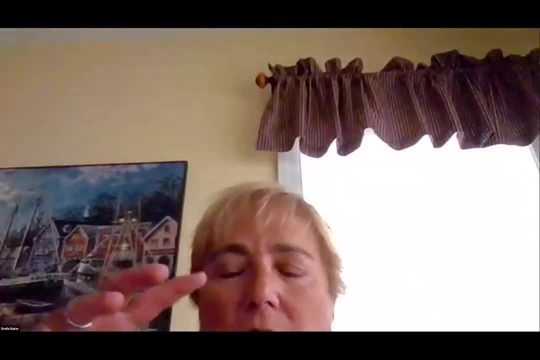 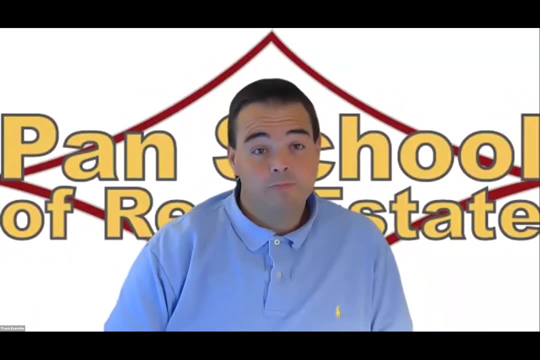 when you were talking it more, it was more about individual owners. but what about, like, community property management? are we gonna talk about that? or you mean like yes, like yes, we don't talk about HOA management. you can manage HOA's with a real estate license, but it's not something we talked about at all. So if you ever want to talk about something that you need to talk about, then go to the website that's on the screen. 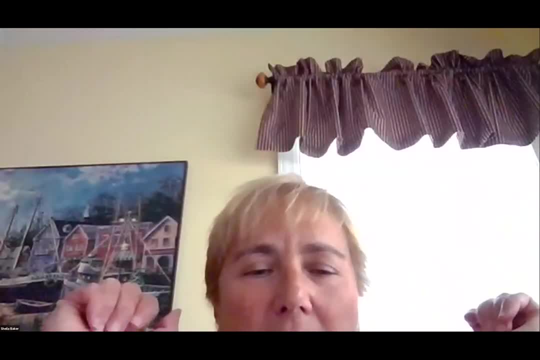 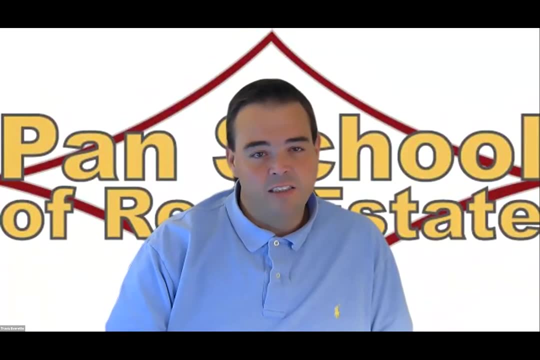 in the course material, So we don't need to know anything about that. Good thank you. Yeah, it's just a. it's such a niche thing that it's not something they put in the in the materials. I'm glad that would be complicated. It is complicated. There's a lot that goes into that. All right, so we're gonna move. 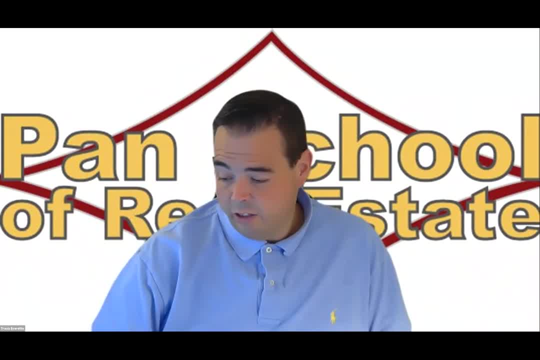 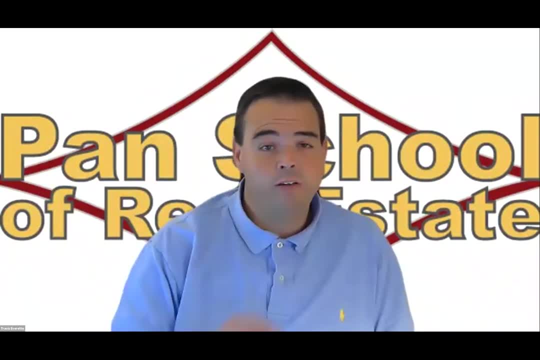 right on to chapter 19 if you want to go ahead and get your slides out for chapter 19, which is the fair housing chapter. And we jump ahead to chapter 19 here because it makes sense to talk about fair housing right after we talked about landlord and tenant and property management. Because I will. 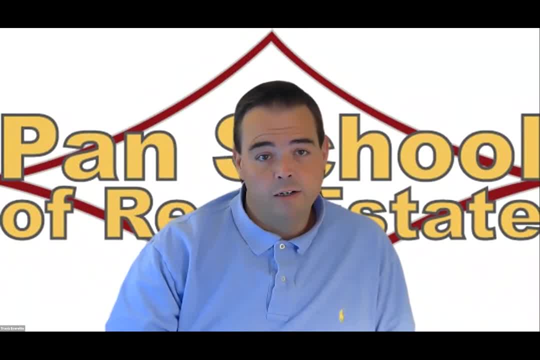 tell you that there are lots of more common issues with rentals than there are with sales when it comes to fair housing issues. And I have- and I just do y'all weirdly, do y'all have like pictures of me in your slides for this chapter. Why are those in there? 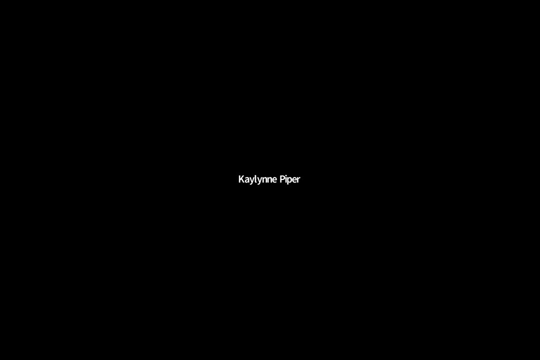 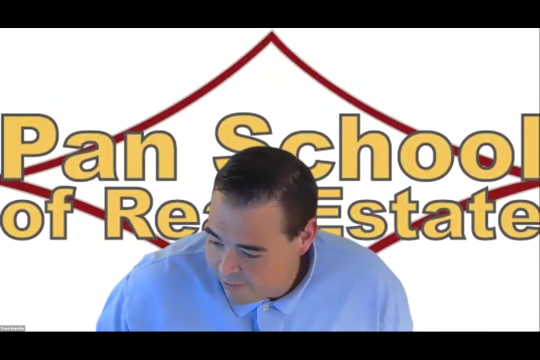 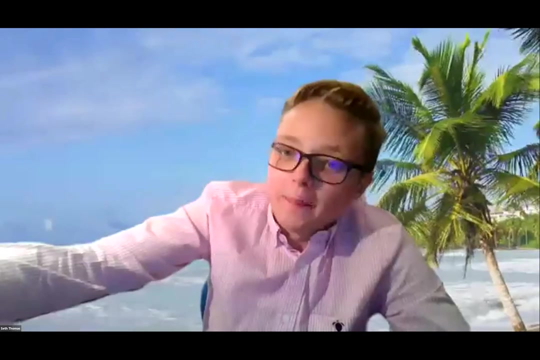 Yeah, yeah, I have no idea why. I thought I might have thought it was fair housing. Well, maybe it was. Maybe I was determined that we were gonna talk about fair housing. I guess I have no idea why those are in there. That's so, Travis, what happens when a business does not? 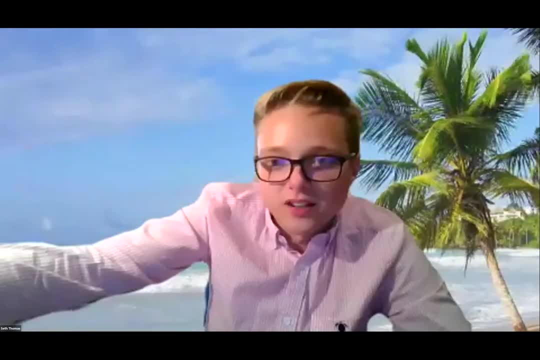 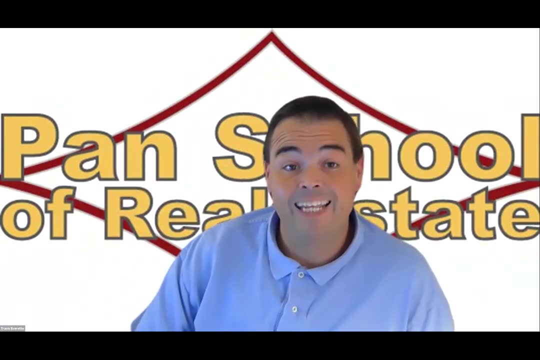 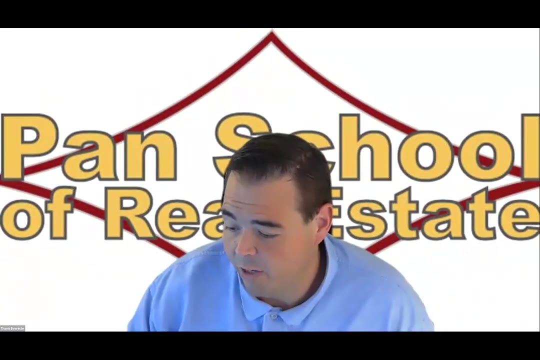 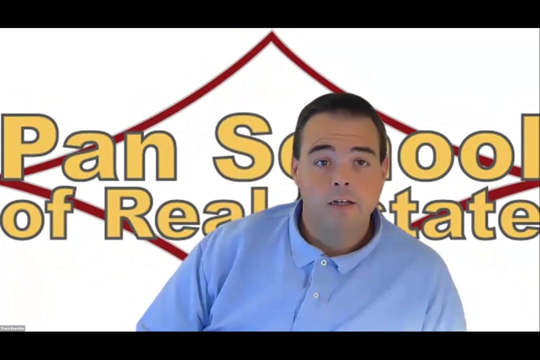 comply with the rules for fair housing. There's several that Brittany can think of that do not have access points for wheelchairs. Who well they? they don't compare. comply with ADA access rules? Yes, Because if they're public facilities they wouldn't have to comply with fair housing. They would have to comply with the Americans with Disabilities Act. If someone were to file a complaint against that property owner or property manager, then if the person is not in the area they wouldn't be able to comply with the rules for fair housing. 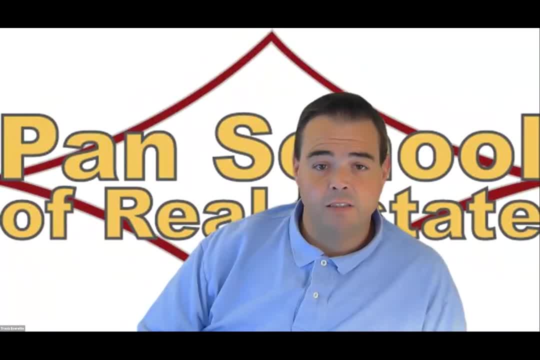 Yeah, Okay, uh, the the united states um, uh, department of hud, housing and urban development uh, which enforces the americans with disabilities act, would come in and investigate that complaint. um, also, the north county human relations commission could investigate that complaint and potentially find either the